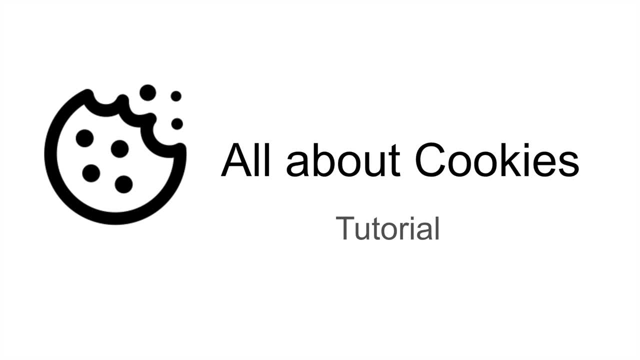 content of this channel. With that said, let's just jump into this exciting topic, right, All right guys. So, so cookies, when I decided to, you know every almost if you ask anyone from the streets, like what are cookies? like what cookies are, obviously, if you tell them that, hey, I'm talking about. 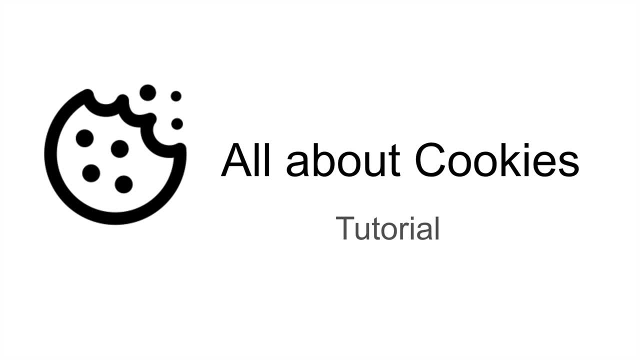 technology here. right, They'll tell: yes, they're on the browser cookies. sure, right, They know right. Most people know what cookies are, but I decided to kind of step out of this bubble and say: you know what? I don't know anything about this And I wanted to learn- almost I want to learn about this. 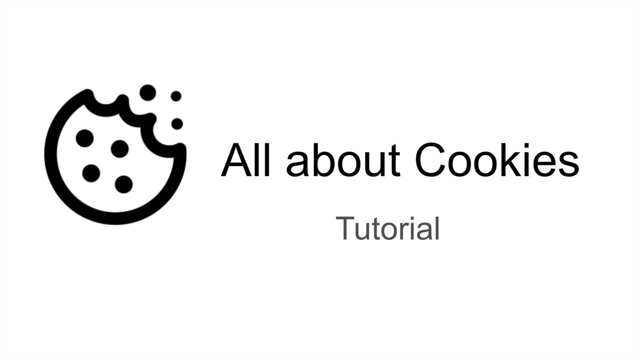 What? what are these cookies? What are all this kind of different things, how they work, right. So I started, I did almost a two week research and I still think I don't know a lot about these things. So I'm going to distill what I learned about this topic here and 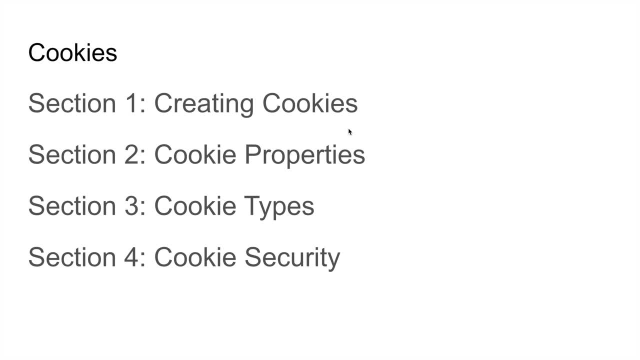 hope you guys can enjoy. With that said, let's just jump into this. So I did. I'm going to divide this tutorial, if you will, into four sections. I'm going to show you how to create cookies that differ in methods of creating cookies. Yes, there are more than one. 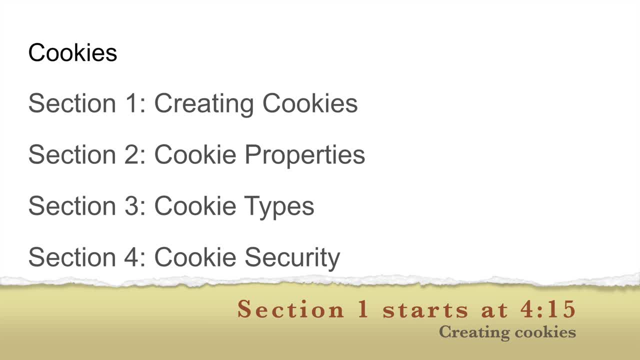 method of creating cookies. right, I didn't know that Right, And yes, most of them like using JavaScript, but there is a server side way of creating cookies and there is a client side way of hearing because we're going to talk about that. So what section two we're going to talk about? 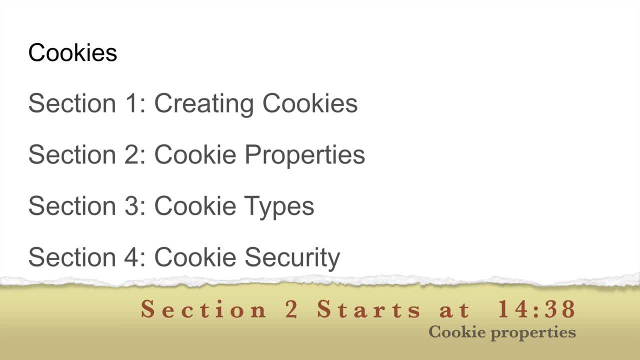 cookie properties, right, and there are a lot of properties for, for, for the, for the cookie there's the max age and expiry in their same site and other stuff as well. that we're gonna talk about, right, and then what, what, how they like, what is the contract of the cookie? we're gonna, we're gonna talk about that. 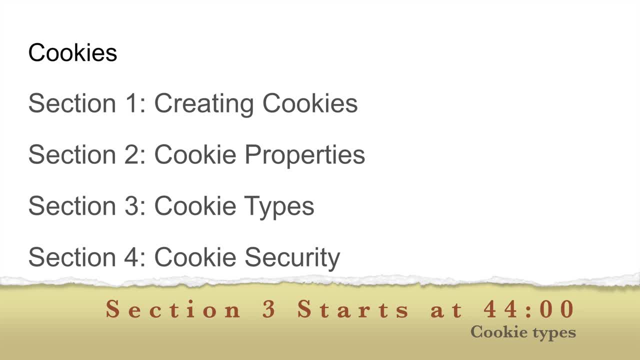 right. so what makes a cookie cookie? it's actually three. we're gonna talk about cookie types. there are a lot of types that are, in my opinion. they're made up right, it's just not ties, but it's kind of of kind kind of like attributes associated to this, to the, to the type of cookies you know. it's like there, there. 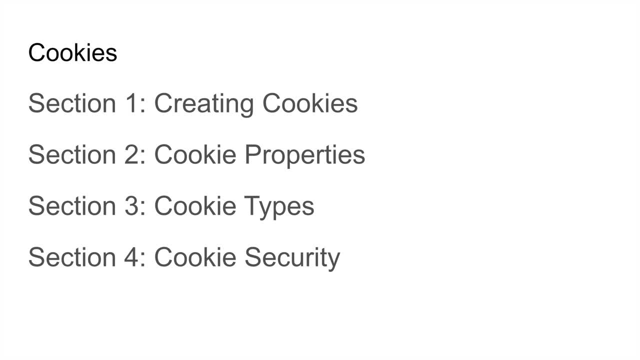 are different types and we're gonna talk about them. they're permanent session based. it should be only. I even included zombie cookies there for you, to for for fun, before we're gonna talk about cookie security, which is insane man. so the way, there are a lot of ways to steal cookies and hijack sessions, I was so surprised. 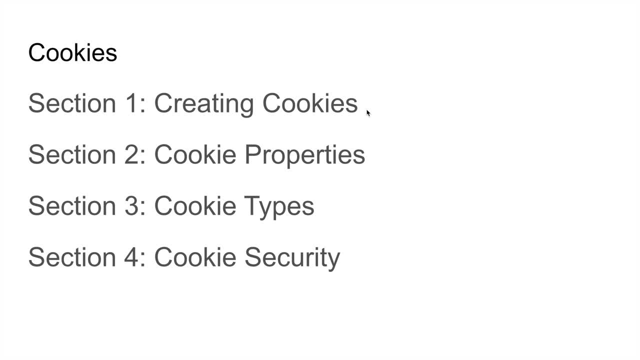 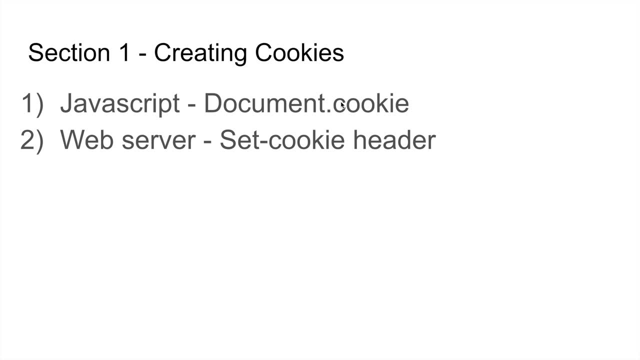 but, but we're gonna have a lot of fun, guys, right? so, with that said, let's just jump into section one, where we will create cookies. creating cookies: okay. so there are two ways to create cookies, guys, right? so there is if you, if you go to any browser right now and you go to googlecom and you open the 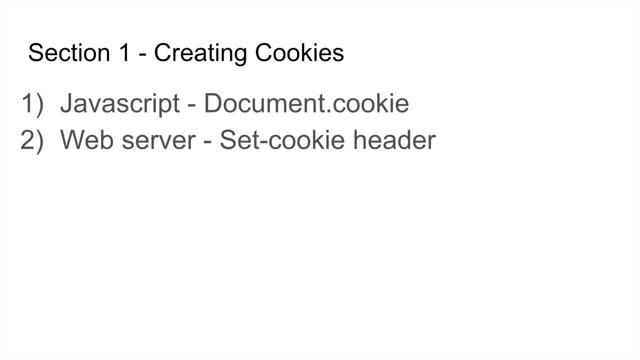 console in Chrome. you can type some javascript there and you can literally do this: code right, document right, which is the document that you open, which is googlecom in this case, and then you say: document dot, cookie equal. something equals, something right, which is the, the value of the key, the cookie, which is. 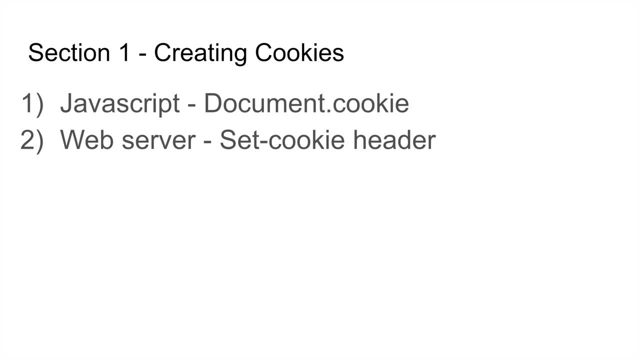 like key value story and you can think of it this way, right, so this is one way of doing this. have a success. once it turns into a pet doing it, you can write a JavaScript code to sit that cookie right. we're gonna show that. and there is another way, which is kind of a server. the server asks the. 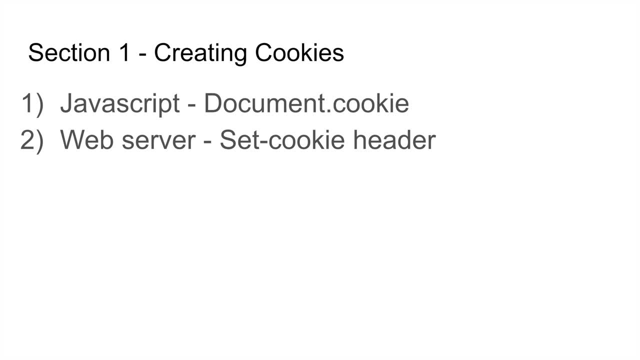 client to sit a cookie for it. so in this case this we're gonna use the header that is called sit cookie. right, and this is a response header. so what happens here? when you make a request to a site, like a get request or even a post request to a site, the site can choose to response with, obviously, the body and it. 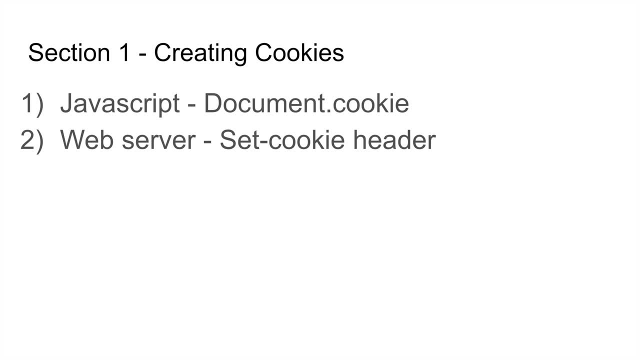 also responds with a bunch of headers like content type, right, and all this kind of stuff. one of these headers- optionally- you can sit a cookie. you can say okay, sit cookie, and there is. you specify what cookie you want to sit and the browser will set that cookie for you and most of the size does that for you. 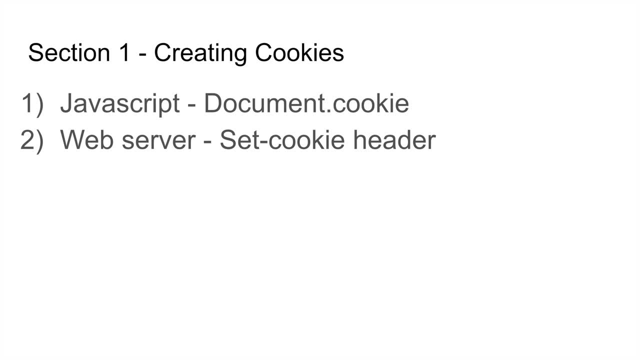 like, if you go to amazoncom ready sign in, it will sit cookie and then we'll return the session ID for you and the browser will set the session, that cookie, for you from that right. so there's no JavaScript involved here behind the scene. browse the browser. does that. it looks for this. 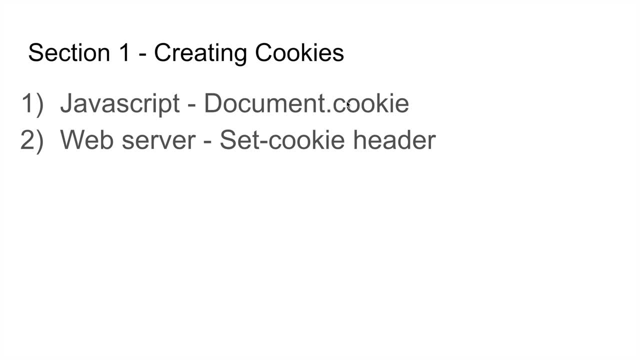 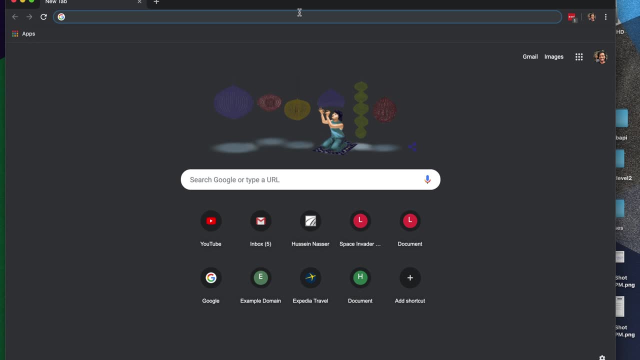 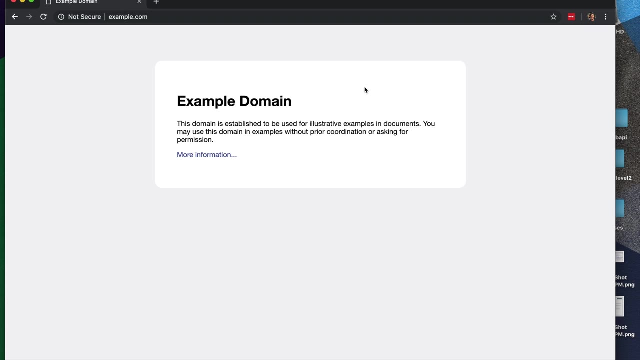 it's cooking and takes that and creates the cookie for you. right, let's just jump and show you both those things. alright, guys. so let's show you one of the ways to set a cookie. right? so let's say I'm gonna go to a site- examplecom- and then 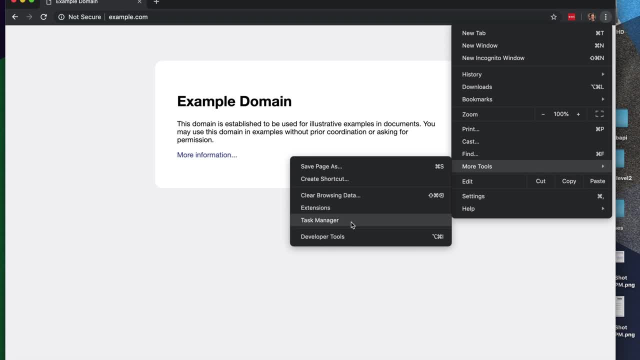 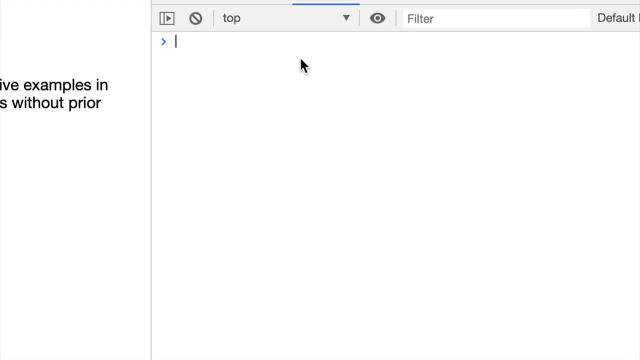 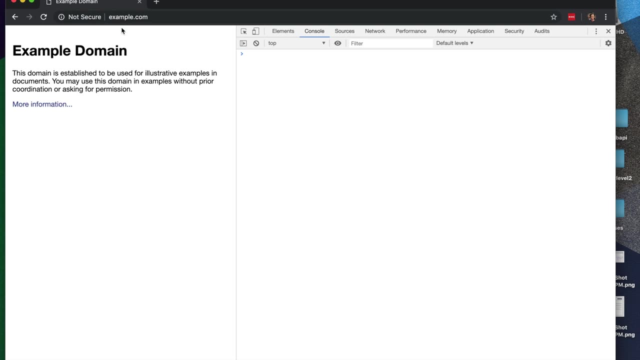 I am going to go to the developer- developer tools here- and then this will open the console which allows me to write some code, assuming that all this code that will be written will be executed in the same context of this domain, examplecom. right, so what I can do is I say document cookie equal. I don't. 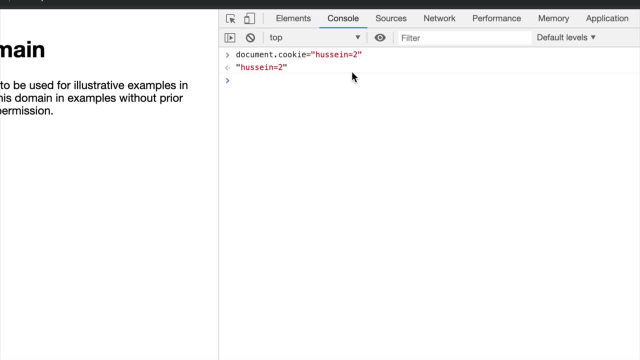 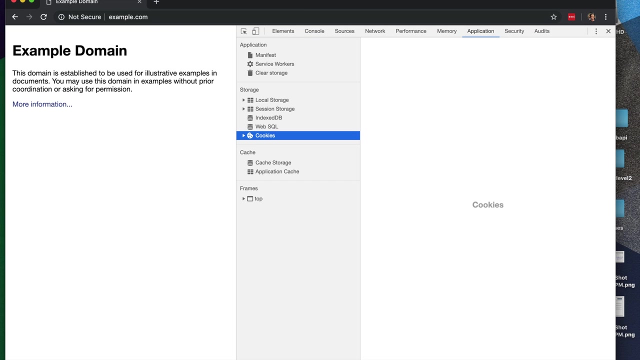 know Hussein equal to right, whatever you can see all the tests that I've been doing right. so now I have set a cookie with the one value called Hussein. the key is Hussein and the value is two. right, and this is how you look at the cookies: right in this domain. we go to the application and then you expand that and 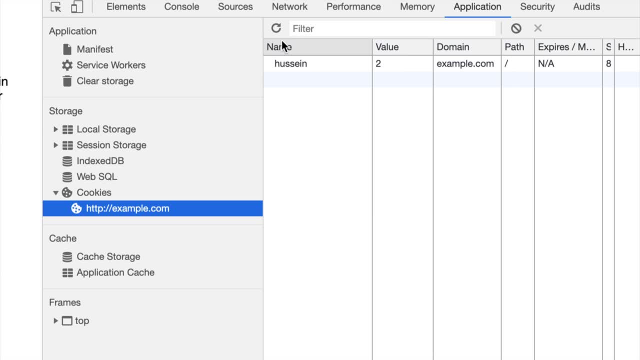 then you can see that there is one cookie named Hussein and the value is two and it's set to this domain, which we were gonna talk about as well. these are part of the properties of the domain, that cookie. so we're gonna talk about all about it, all that cool stuff, right? 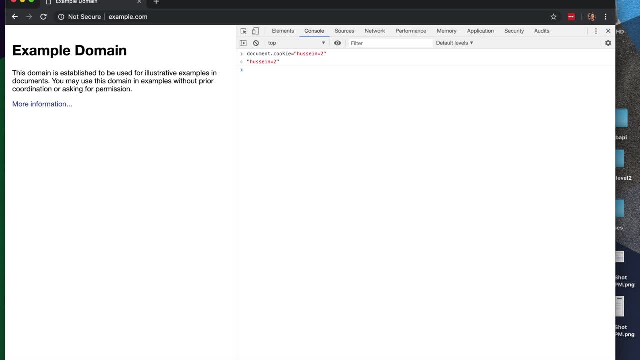 so that's, that's one way of doing it right. so this is the JavaScript way of doing it right. so another way of the kind of the javascript II way of doing it. but let's say I want to build my own website, right? so I'm gonna go ahead and 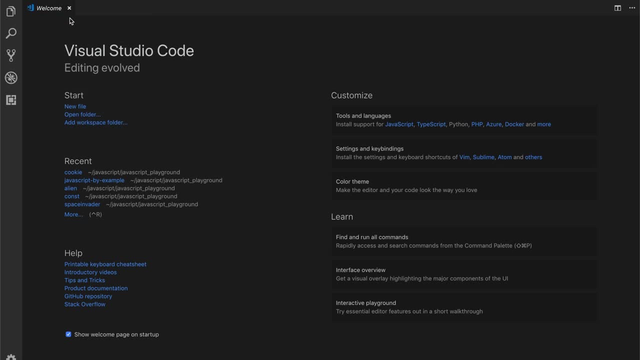 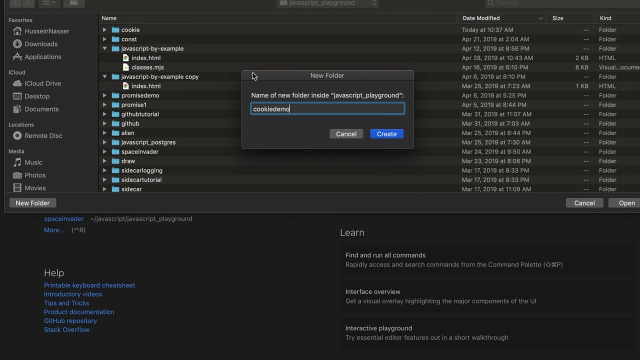 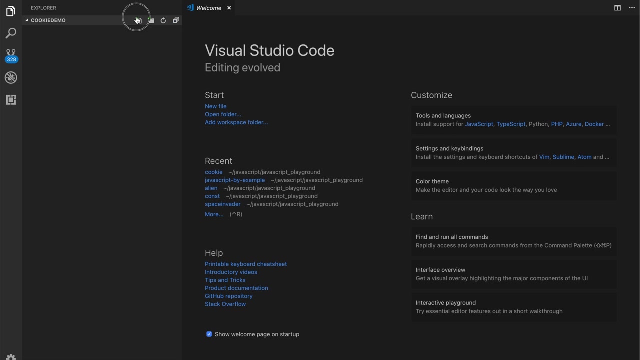 open Visual Studio code here and I'm gonna create a brand new folder. let's call it cookiecom program. and I'm gonna create a brand new folder. let's call it the cookiecom program demo. right, and then what are we gonna do, man? what we're gonna do here is we're 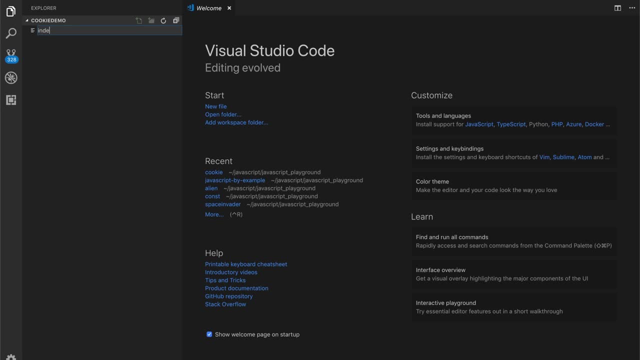 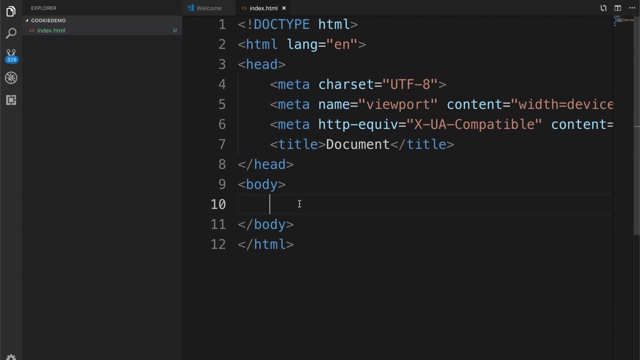 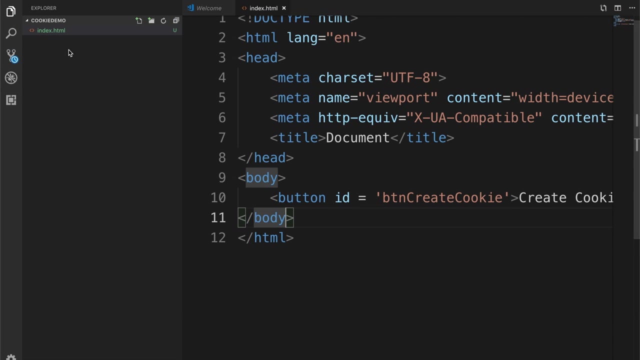 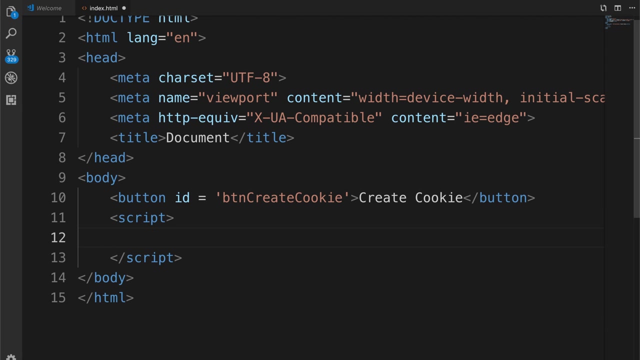 gonna create a new file, indexhtml right and html5, and let's say I am going to create a button here- button create cookie right- and then say create cookie and we'll add some script here and let's say the script will be cons. button create cookie. equal document: dot. get element by ID. 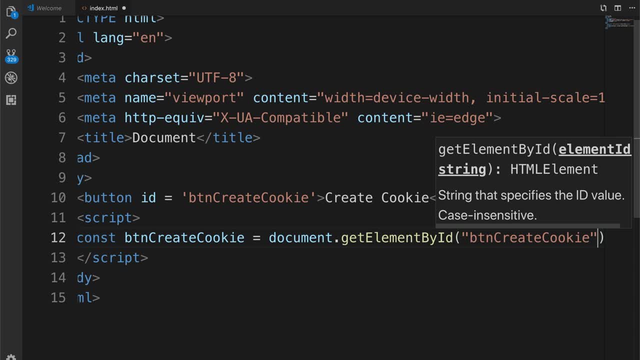 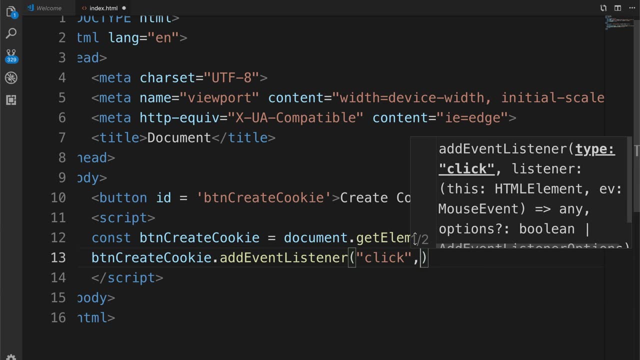 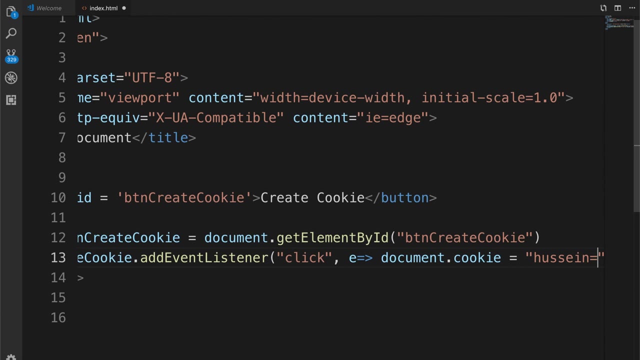 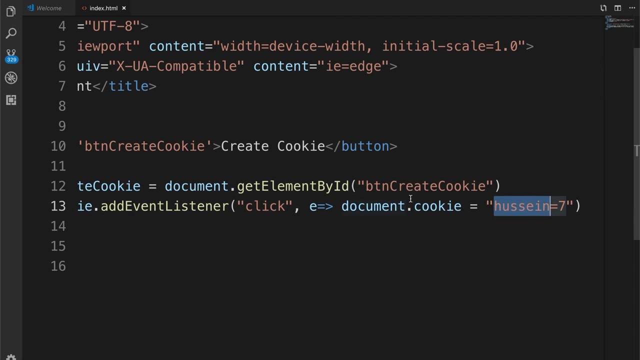 what we're gonna do here essentially, guys, is we're gonna add an event listener so that when I click on this button I want to create a cookie, right. so let's say I'm gonna do document here, dot cookie equal Hussein, equal 7, whatever. it's a very basic cookie, that's. the key is Hussein, the value is 7, okay. 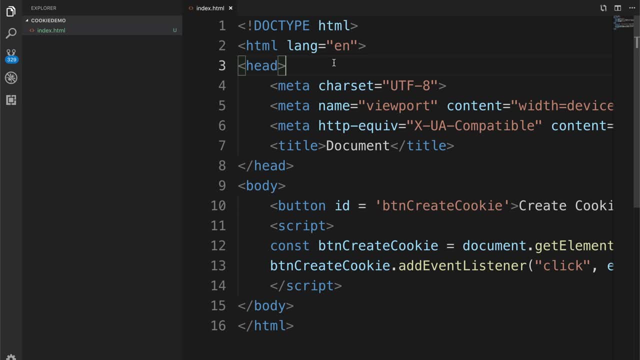 so that's another way of doing the cookie here. all right, now that we have the indexhtml5 right, we're gonna create a new file, indexhtml5, and let's say: ready for us. okay, what we need to do is create an indexjs file and that file. 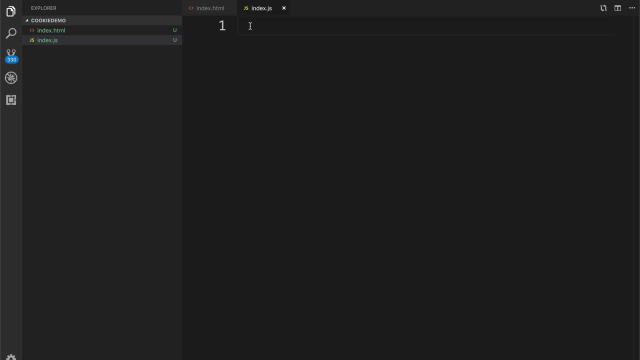 will have basically an express application, a small express application, nodejs application that will return that indexhtml file. okay, and the reason we do that is we like because we want a raw web server that we can control, and Express is great for that. okay, I'm gonna reference the video. 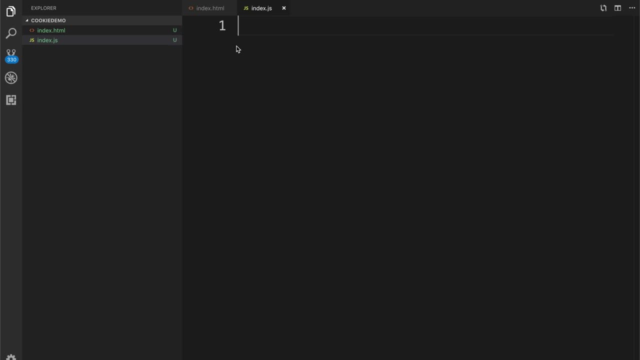 that we did on Express guys. I mean how to install and all that jazz. all right. so here's how we create an Express application- cost app equal, require express. and then you do that. I have express already installed, so I don't have to worry about it. and then what we're gonna do is leicht. 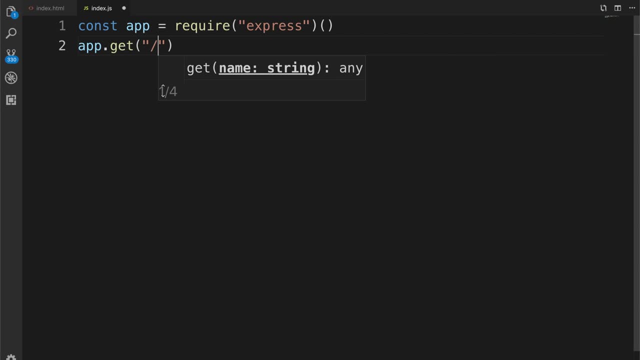 if someone made a request on the route right, I want to get take the request-response function and I'm gonna return the file. that is called direct similaritiessrcop's code- sécuritésrcop's- code.086.086. you can create this app using WCAG or software cameras. all right, now and let's see how this works. 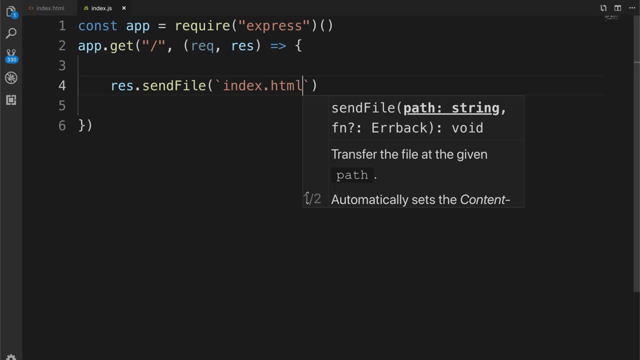 indexhtml all right, but we cannot return it this way. right, we have to specify the path of this and that's the security, just preventive mechanism. okay, so we can do that directory name is the current directory, right, and we can do that and then just add indexhtml. and these are the texts, the beautiful. 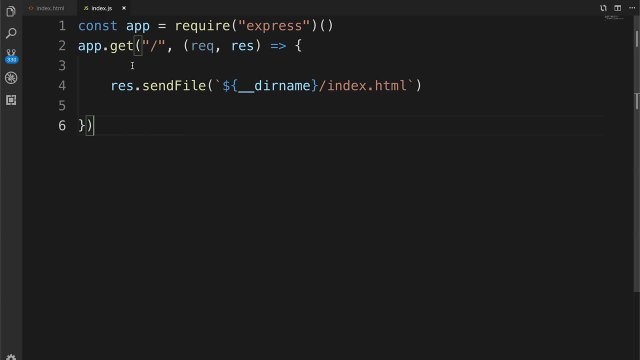 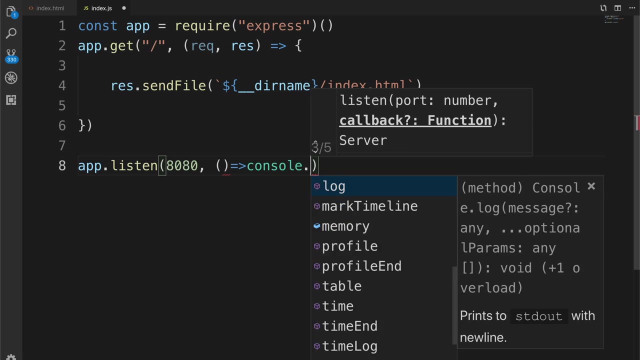 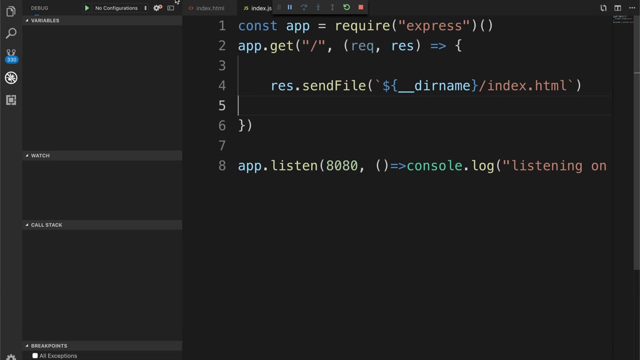 text in JavaScript. this is a new stuff, all right, so now we're gonna send it back, right, but we have to also, obviously, to listen to the to a given port. right, gotta listen to a port in order to satisfy anything, right? and and yeah, consolelog listening on port 8080. okay, let's go ahead and run this thing. 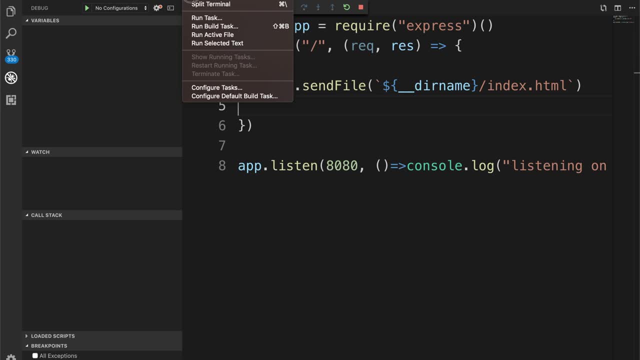 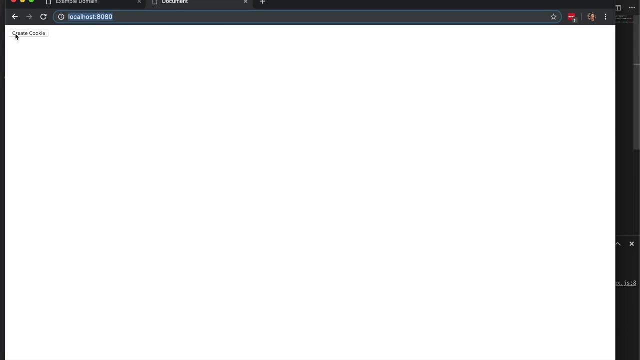 let's make sure we don't have any errors. looks good listening on port 8080, right? so let's go ahead and go to my application: refresh, refresh. there you go. we have our button. there you go, guys, create cookie. so now, if I go to the 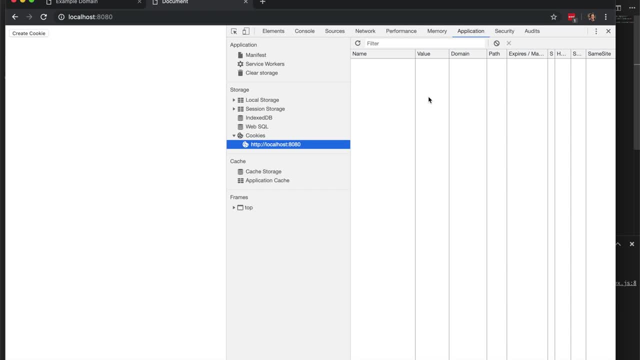 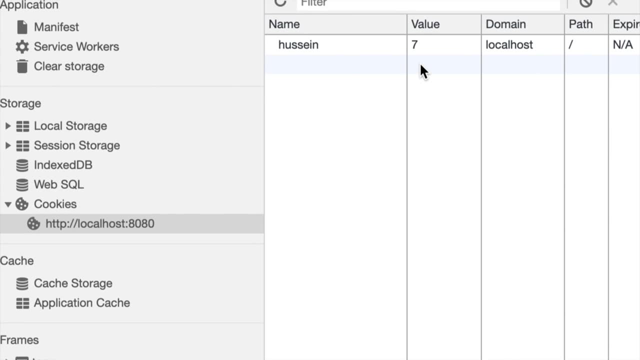 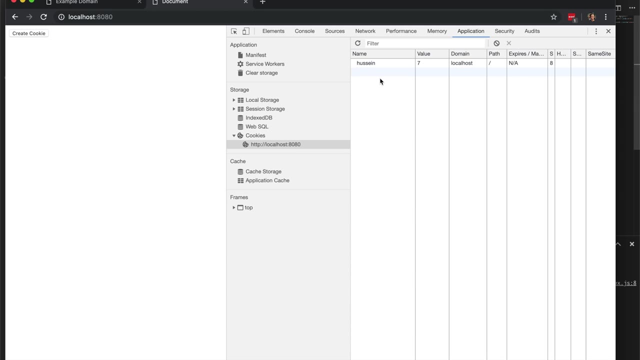 console I go to applications. you can see that I don't have any cookies here, right. the moment I click on this guy, I refresh and we have Hussein seven, right, and the domain and all that jazz. okay, that is pretty cool, guys are. so that is another way of creating the cookie from JavaScript. however, how can we let the 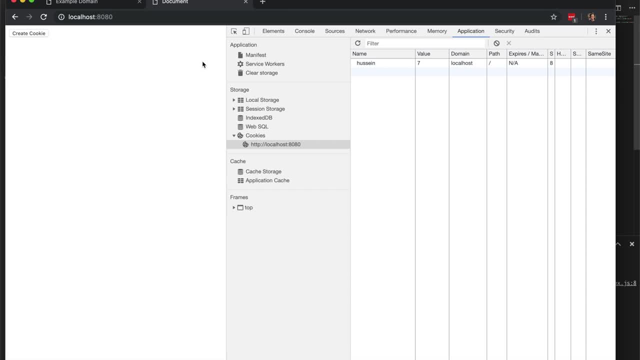 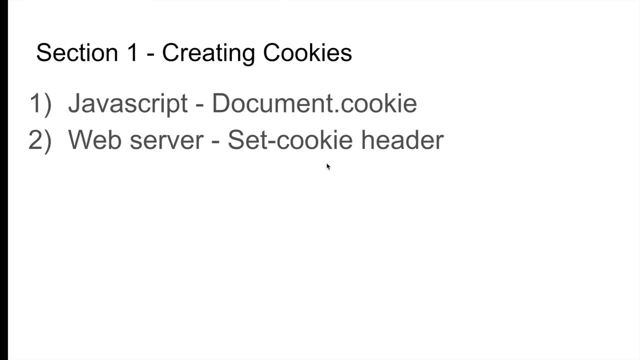 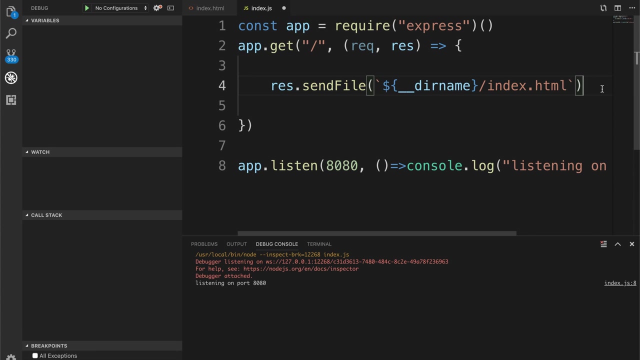 server create a cookie for us without us writing code. okay, in the client edit. here's how we do it. you go to my application here And before we send the file I will say: it's like: hey, if someone visits indexhtml, let him send a cookie. 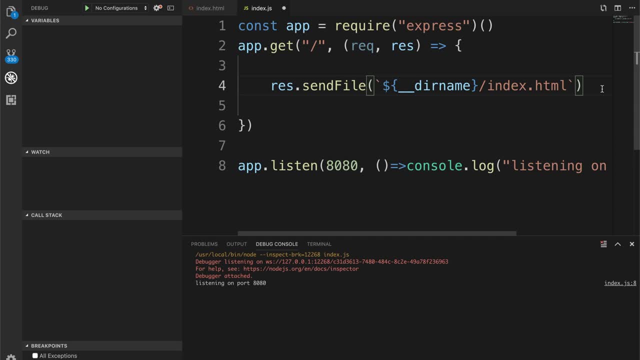 Send that cookie for him. okay, And that's the cool part, You can do it with images, You can do it with indexhtml. It's like cookies cannot. cookies are assigned with anything right, With literally anything. It doesn't have to be an HTML or text or anything. 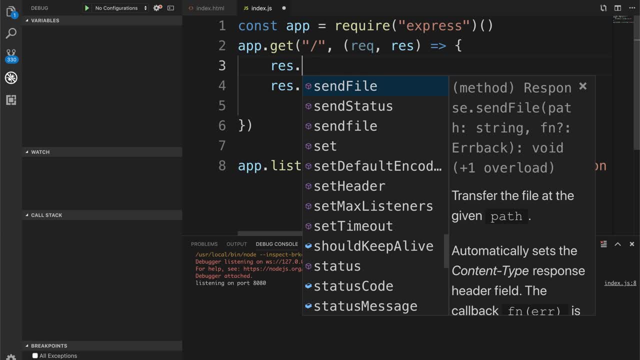 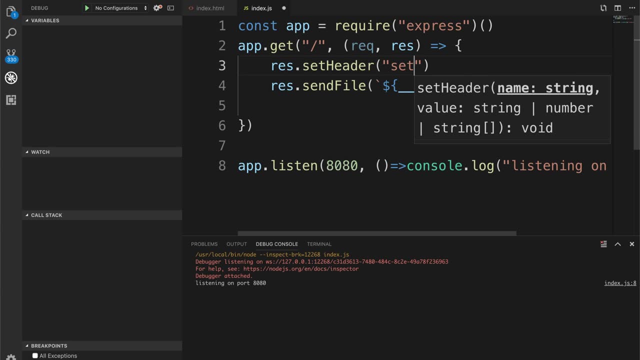 It can be literally anything. Okay, now, when you do resourcesetHeader, you can do that right, And the header name is called setCookie. okay, And here's what you pass. You pass an array. okay, And you pass an array of cookies, right. 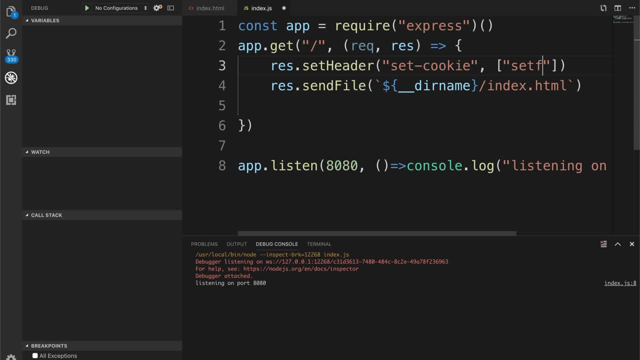 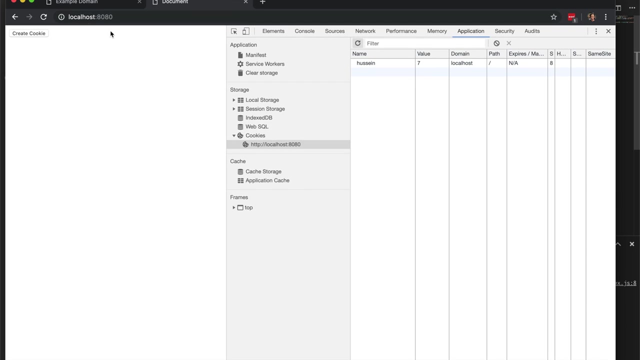 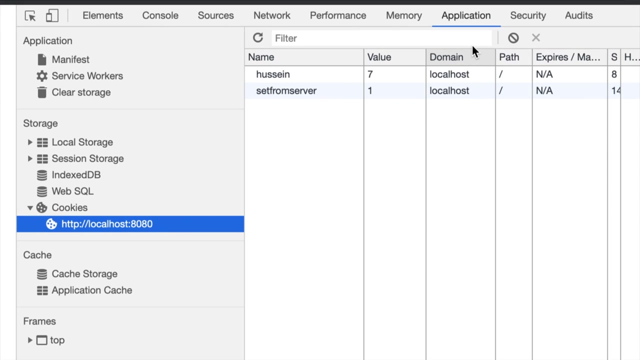 Let's say setFromServer. This has been setFromServer and equal one, right? Let's try this Now. if I refresh this guy, if I go here and I refresh this guy and I go back, look at that: setFromServer. 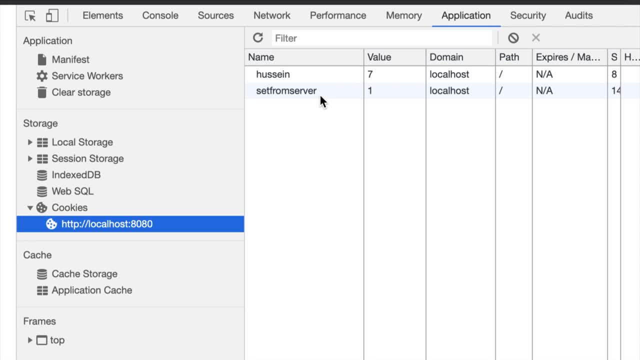 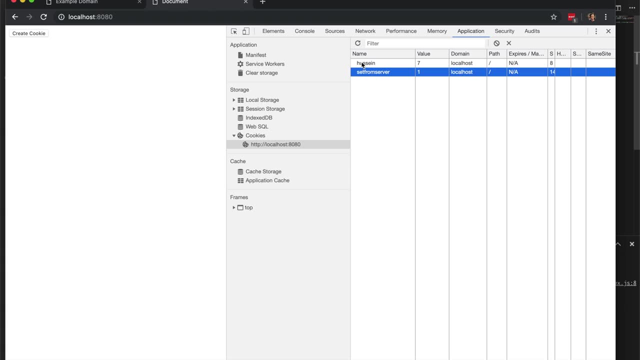 I did not write any JavaScript code yet I have a cookie by just visiting this thing. All right guys. so this is how we set cookies. There is a way from the client and there is a way from the server, right? Okay? so the server sets. 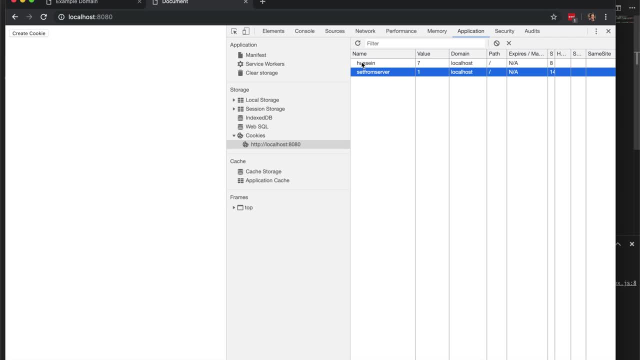 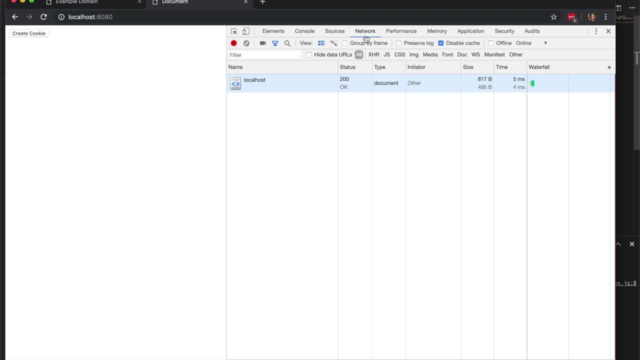 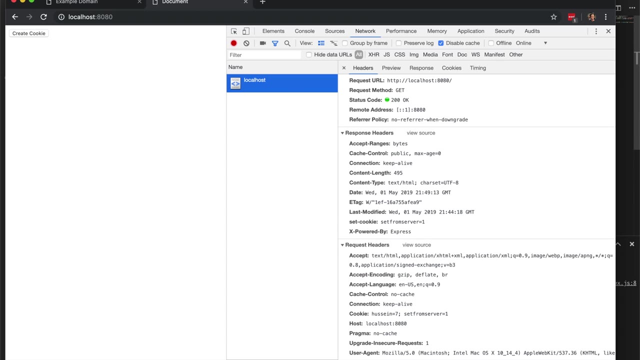 It tells the browser to set the cookie. And let's go and actually check that out, guys. okay, So if I make a request here and I go to network, you can see the request we made to localhost, And if we scroll all the way, we're going to talk about that next right. 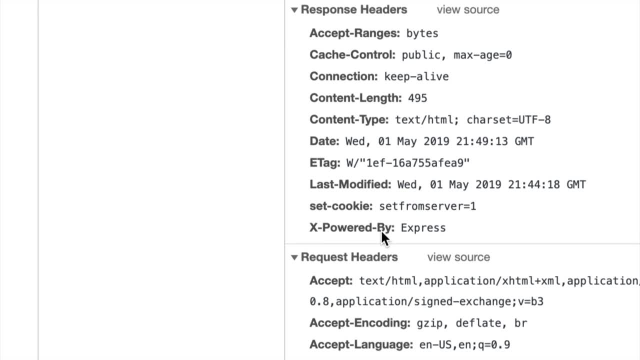 But this is what we're talking about, guys here. See: Okay, setCookie. The browser has been asked To set a cookie from the server, right, And this is what the server is powered from, right? So all the response headers: this is what we're looking for. 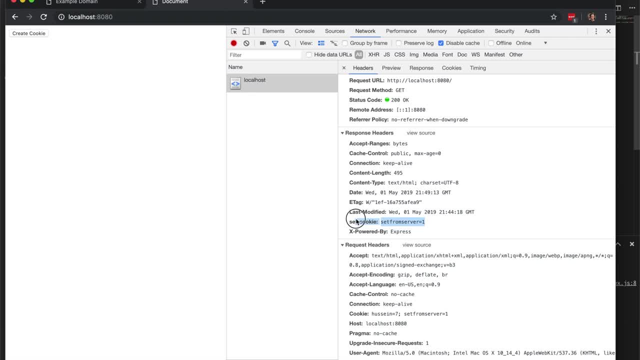 setCookie, setFromServer, equal one. And now, every time we visit this page, we were asked to set this cookie. okay, And this cookie is called the session cookie, which we're going to talk about as well, Because it's kind of temporary. 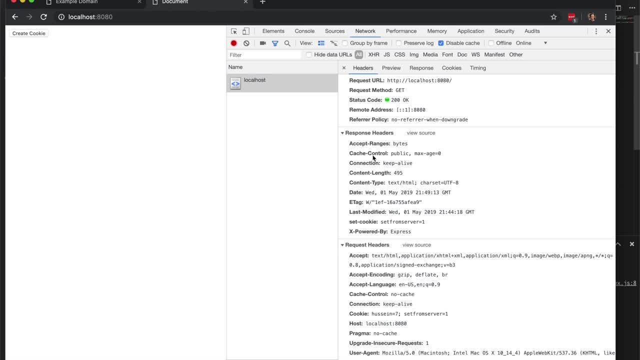 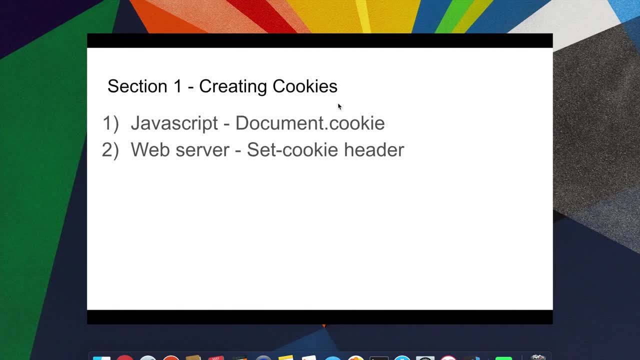 The moment we close this, it's all gone. All right, guys, All right. what do we have next? We learned how to set a cookie From the browser and from the server. What do we have next, guys? Cookie properties, guys. 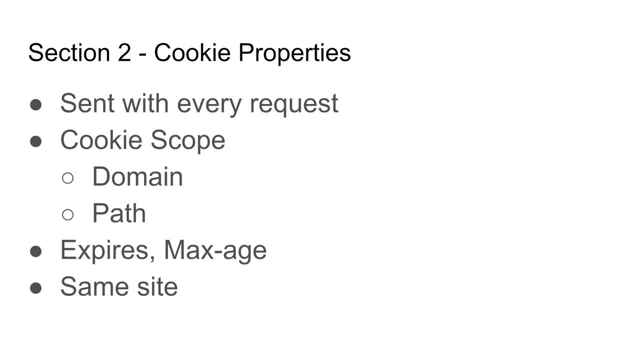 All right cookie properties. So here's something about cookies that you need to know. right, And cookies are sent with every request, whether you like it or not. There is an asterisk after that, But cookies are always sent. There are some cases that cookies are not sent. 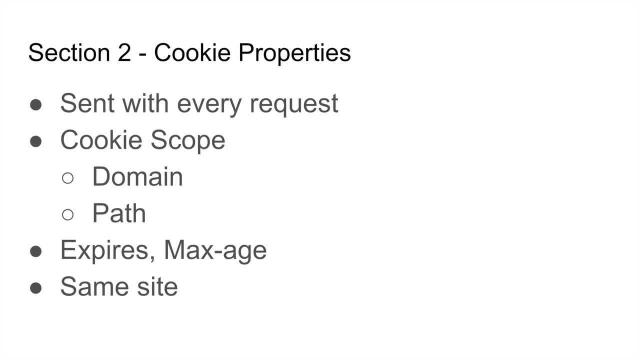 And these are like kind of security things that we can come to, But they are sent with every request. If you visit a link, if there are cookies sent to that domain, it will be sent with that request, right, And you can think about it right. 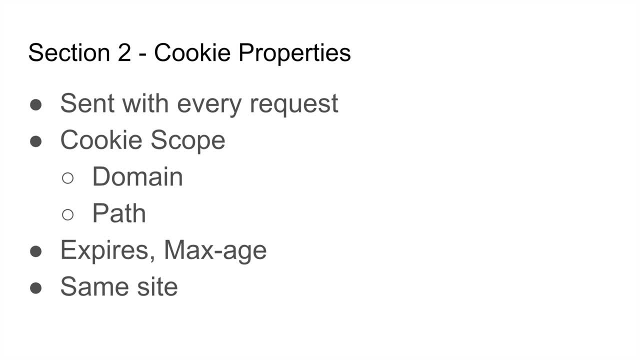 Now, oh my God, What if I have like thousands of cookies? I'm just now sending all this, All this bandwidth right, Just like all this kind of. all these cookies are sent with all my requests. If I visit a link, if I made a fetch request, if I made a post request, these cookies are sent if there are any right. 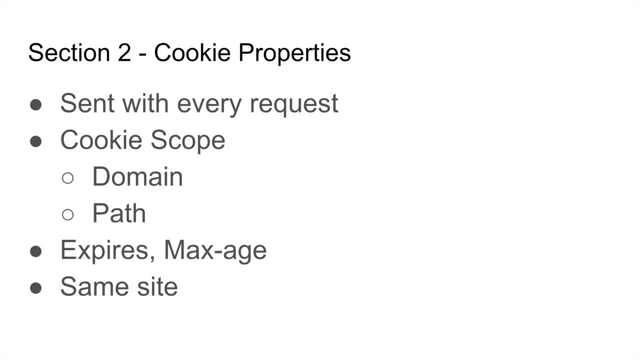 Assigned to my domain. okay, Which is my next topic. here. There's a cookie scope, right? So remember, when we did the first thing, We did an examplecom And we said: the cookie here, Cookies are. think of these. cookies are like buckets, right? 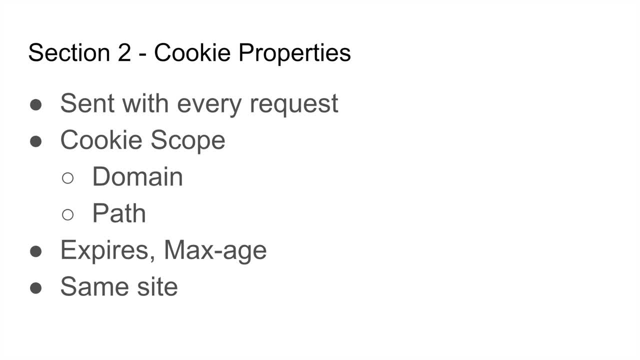 Each cookie has, like each domain has- a bucket right And the cookies goes into this bucket right And this bucket is called the domain right. So if you go to examplecom, literally examplecom, I didn't say wwwexamplecom. 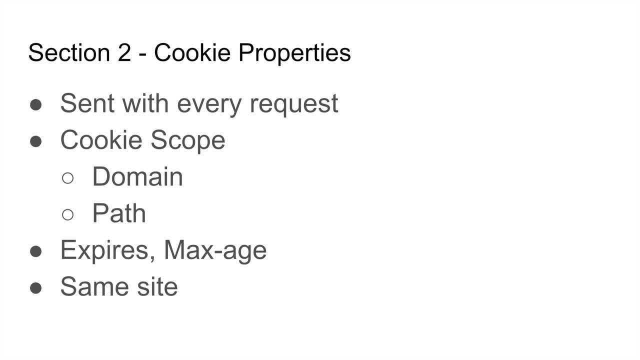 That's a different domain. If you go to examplecom and the server sets you A cookie, that cookie goes only in examplecom bucket. If you go and do documentcookie and you set that another cookie, that goes into the same bucket, and so on, right. 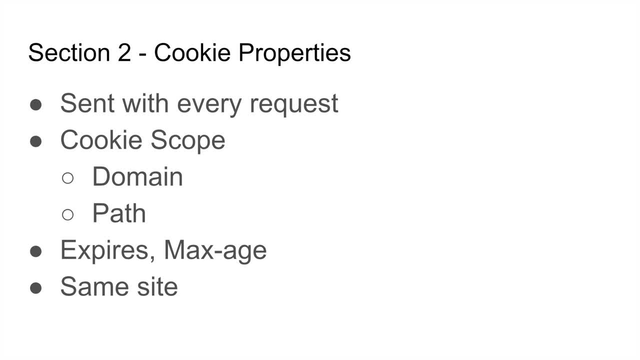 So, in our case, localhost 8080 is another domain that goes into a bucket right. Any cookie creator will goes into this bucket right. So this, this is the path of this, This is the. this is the scope of the cookie domain right. 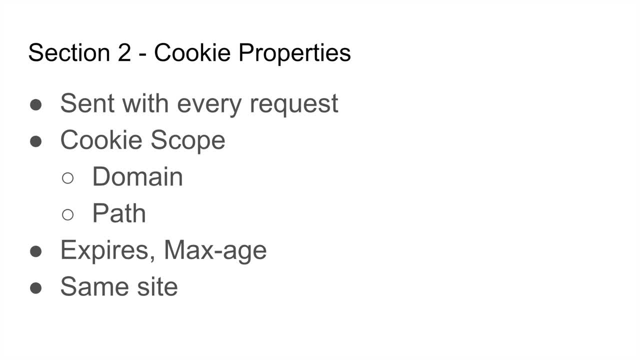 And the second one. The second one is the path there are optionally, you can set paths for the cookies. all right, you can say, for example, I want these cookies right. Let's say you have. you have examplecom right. 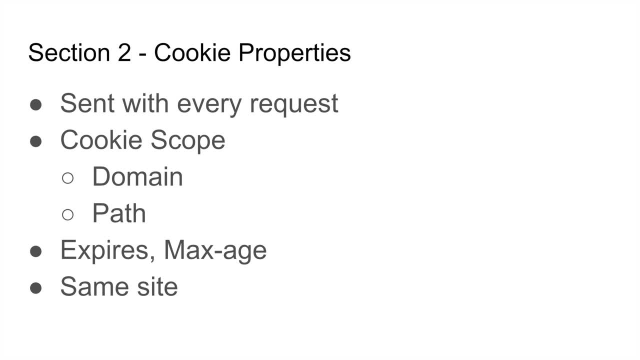 And you have. you have a lot of cookies, right, But you want- you want some cookies to be sent to certain path, like slash login, But Other cookies do not send it to this path. send it to other path, right. 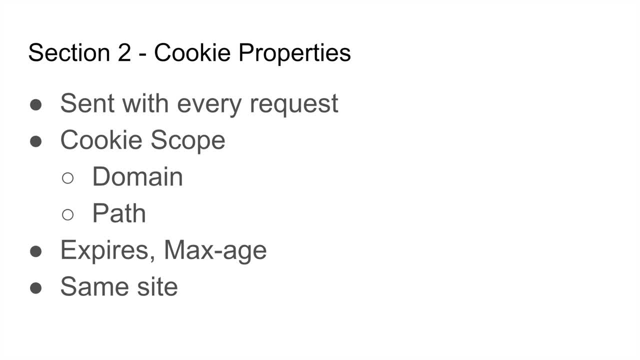 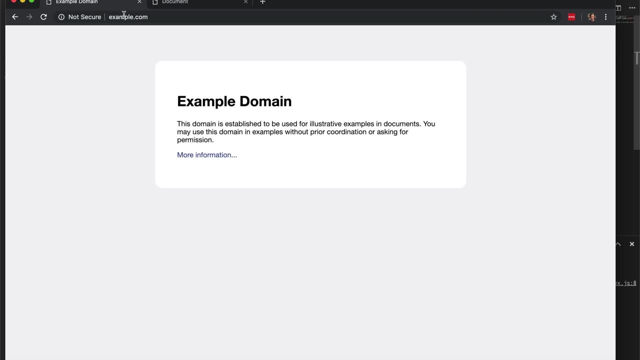 So you can specify cookies per path as well. We're going to talk about that. So as a let's just jump into some demos guys here. Domain. All right, Let's go back to our example here. I like this a lot. 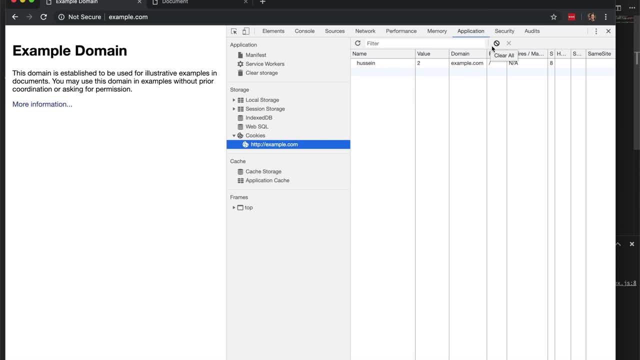 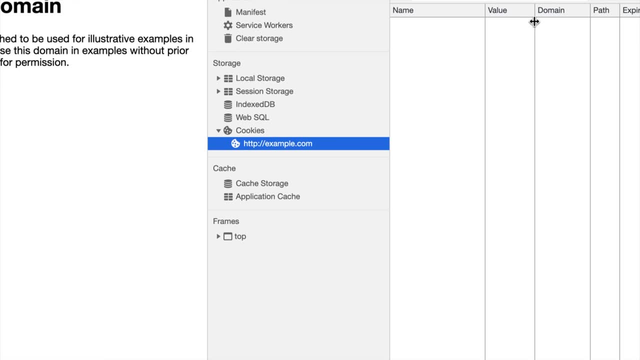 So go here. Do we have any cookies? If we have, let's clear them out, clear all the cookies. and here, here's what we're going to do. We're going to go to examplecom And I don't. I don't have any cookies right now. 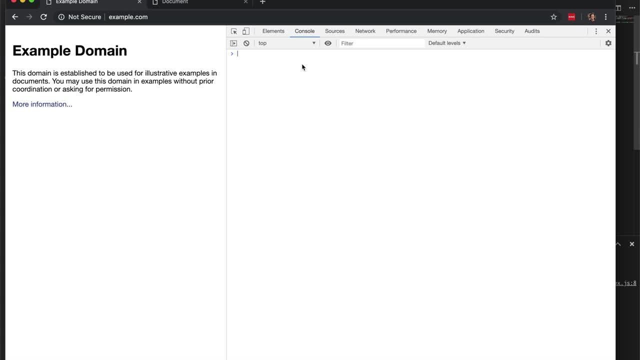 Okay. So what I'm going to do here is I am going to create a cookie, Okay, And uh, document dot cookie equal, let's call it um. I was saying: make one one, Okay, And obviously when you refresh, 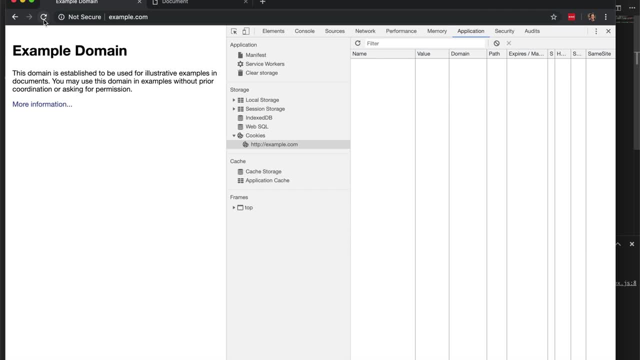 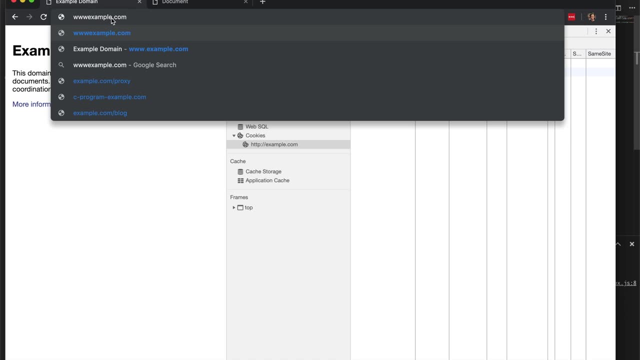 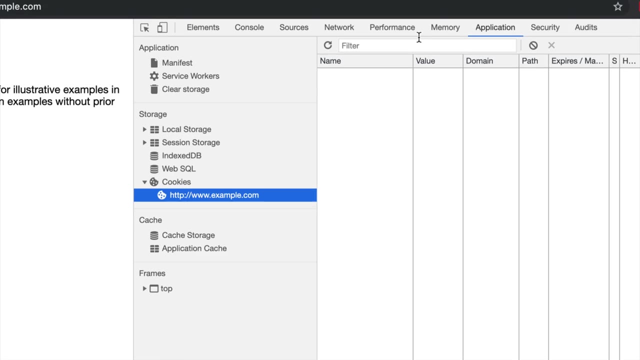 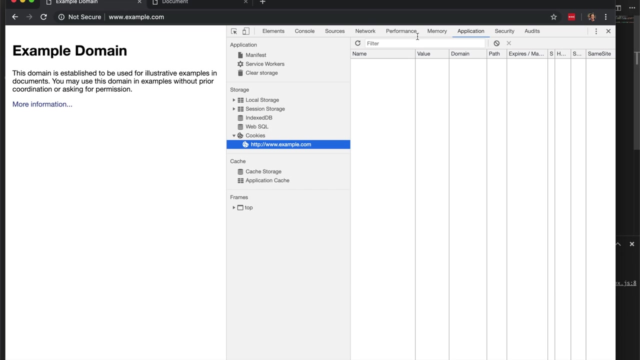 There's your cookie, a great an examplecom. Okay, Now, if I go to wwwexamplecom, guys guess what? My cookie is not there? because that cookie that I have created was, if I, if I say document equal, Hussein, equal one, that default. 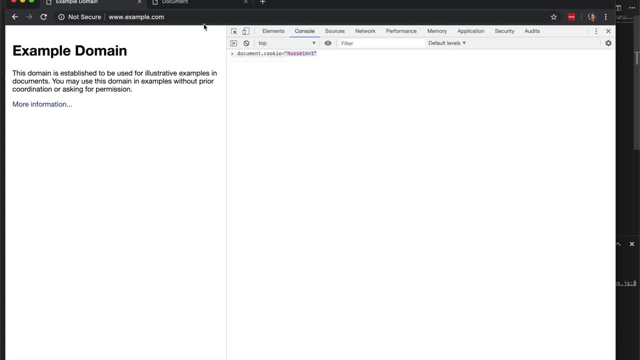 Is it only is created for that particular domain, which was examplecom, and that's it. Nobody else can see it. Not about that. examplecom, not mailexamplecom, not wwwexamplecom. These are different domains, right? Obviously not googlecom. can't see it. 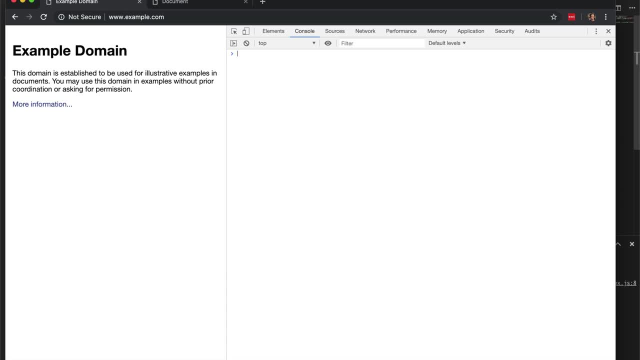 All right, So by default, if you create a cookie like that, it will only be seen for that particular domain, right? Okay, So now if I have, uh, if I create- let's like create a cookie for this guy only, okay. 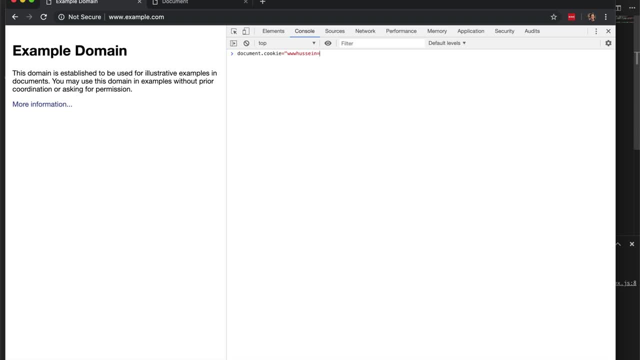 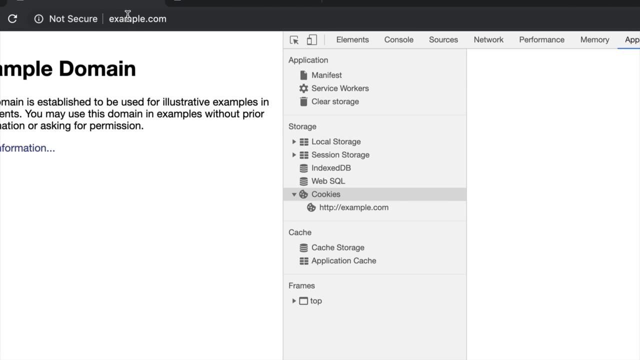 Equal w w w the same, equal one or two. Now this guy, I can see it right. Refresh Sweet, I can see w w Hussein. If I go to examplecom, I better not see the w w one right. 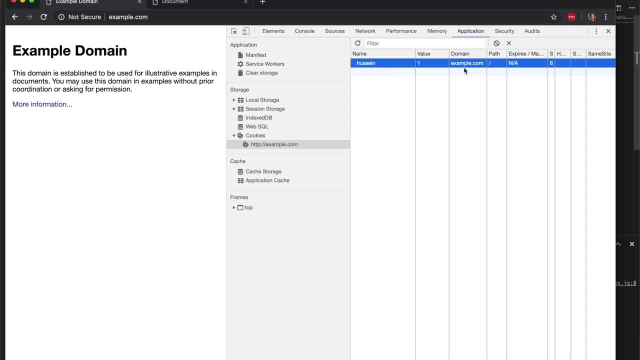 So I can see only this guy, Right, Hussein. Okay, And it said the domain is examplecom. If I go to w w w- examplecom, you can see that I can see the other cookie. right, So cookies are paired domain. 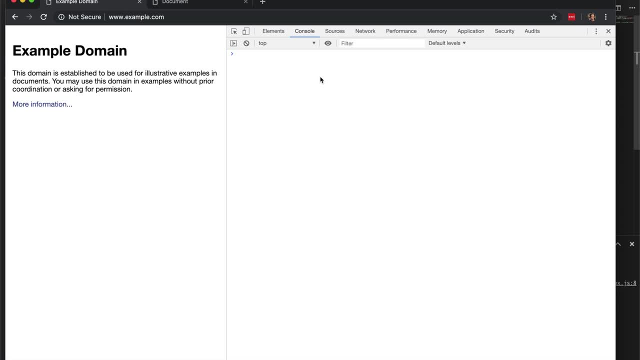 However, you can specify a property for the cookie that is called domain. And guess what This property is? All those saying, let's go, I'm going to create a all Hussein. but I'm going to add a property to this cookie called domain, and I'm going to specify just dot, examplecom, which means that says: okay, this cookie please make it available on all subdomains: examplecom, w, w, examplecom, aboutcom, mailcom, anythingcom. 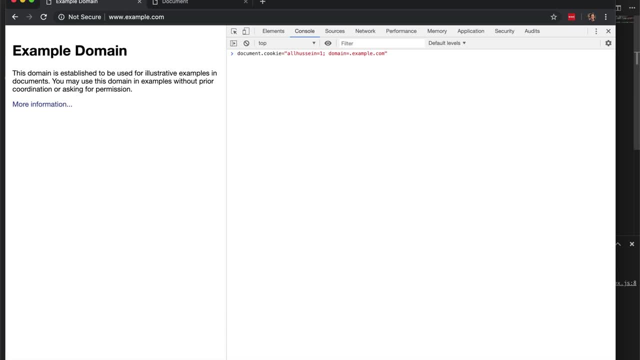 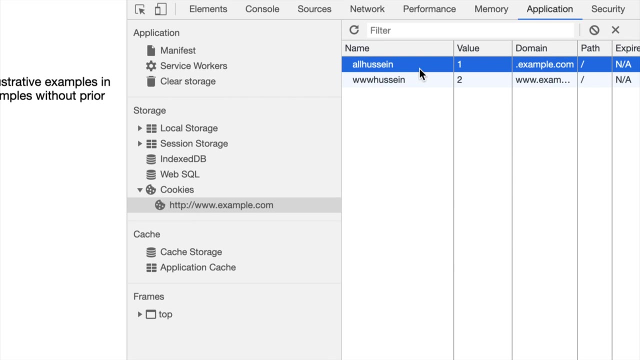 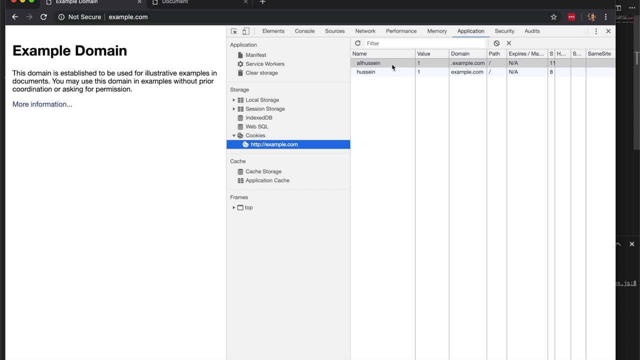 Right, And make it available there. That's what this means. Now, if I do this, I go to application. Hey, I am in w w. Obviously, I just created here, right, All Hussein is there. If I go to examplecom, I also see it here. 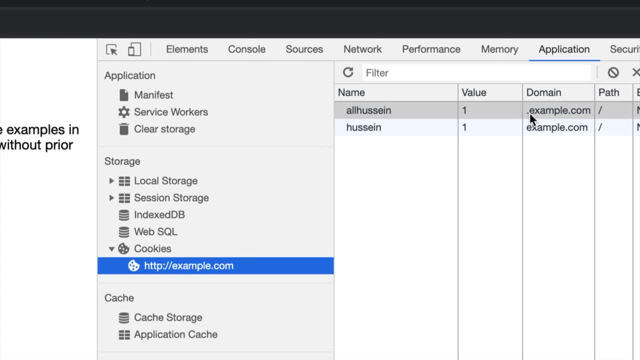 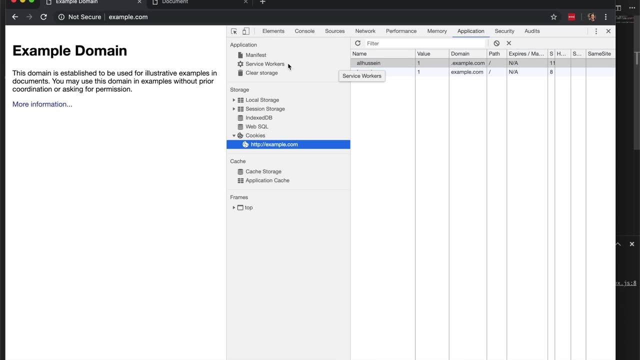 Isn't that pretty cool guys? And see the domain right: Dot examplecom. right. It's different. Not examplecom is dot example. That means everything, everything in there. isn't that cool-ish guys? Isn't that pretty cool, huh? 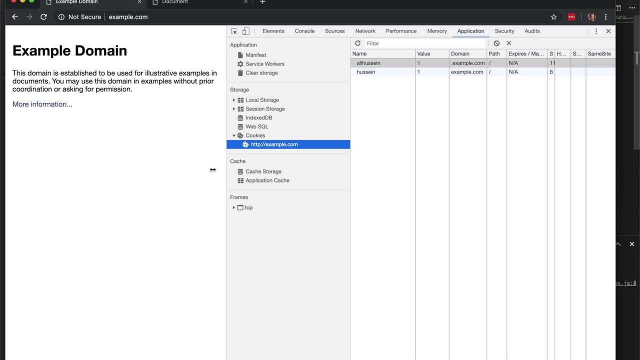 So that's cool, The verge, I don't care. All right, So we're on about the domain. So that's all all we need to know about the domains, right? So the we, we, we, we need to talk about cookies and sending them. 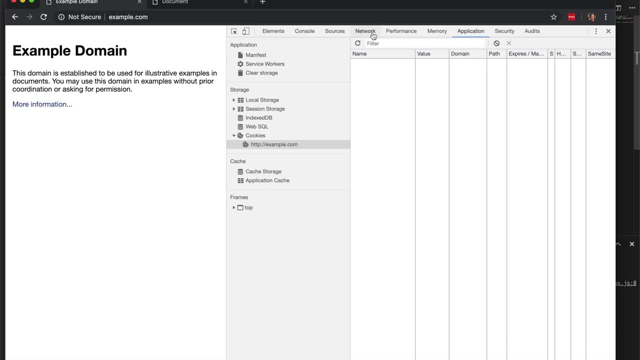 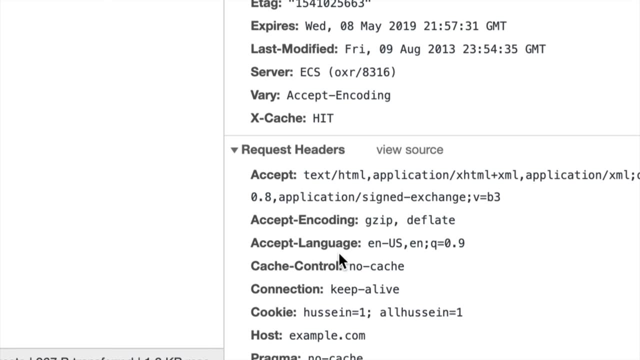 The cookies as well, right? So now if I go to examplecom, let's go to network and see the request that I made, example that come enter made a request, right, And look at that. guys, we're sending the cookie. 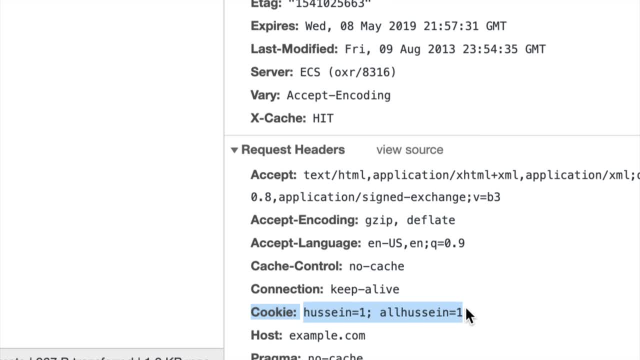 We told them we talked about this. right, We always send the cookie with every request, cookies that are relevant to this, uh, in this case, uh, to this domain, which is examplecom. I have a same, equal one, and all who are saying that one which is this one is available to all subdomains. 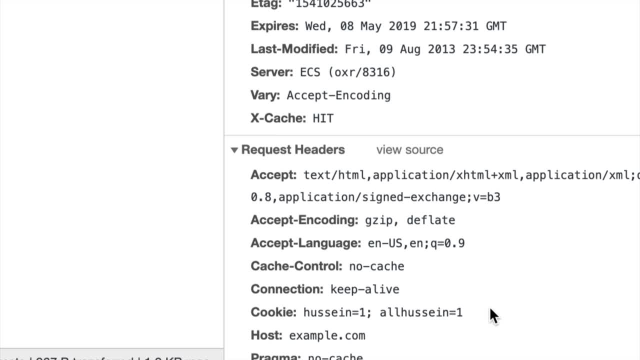 So we get this cookies, So we always send this coach, So the server has it. It was if each request- because, remember guys, HTTP is stateless, So it gets all cookies Every time. you have to send as much information as possible, right? 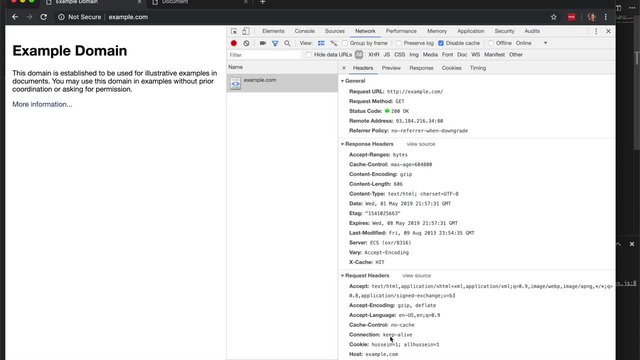 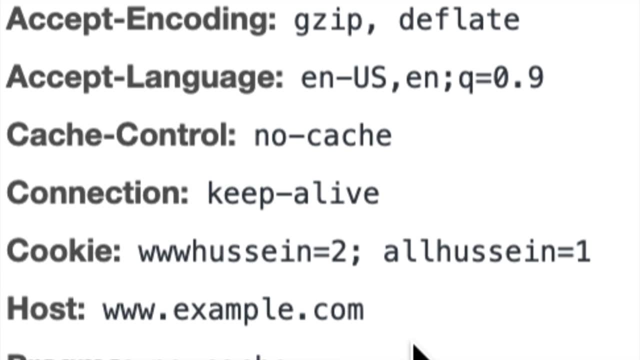 Because the server doesn't store anything, All right. So if I go to WWW and I go click here, You, we get this different set of domains guys, different set of cookies, but that's, that's what we're talking about, right? 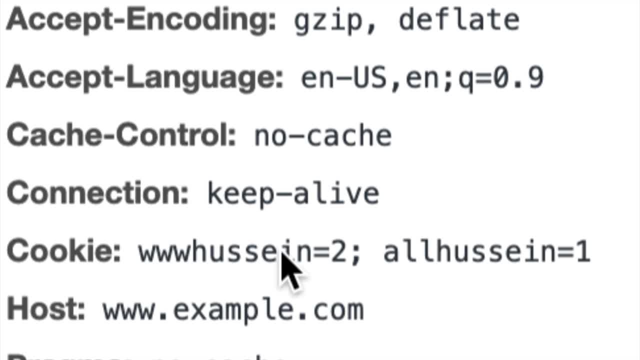 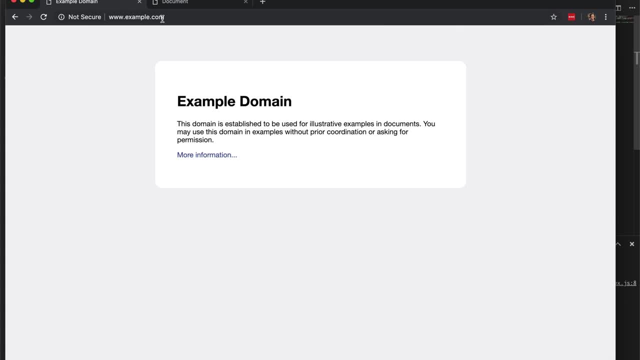 We get always. we send the cookies, right. That's a different. that's the the other cookie we talked about. All right, And uh, let's go back to our local host If we still have that. Now, if I go to developer, let's make that request again. you can see that. 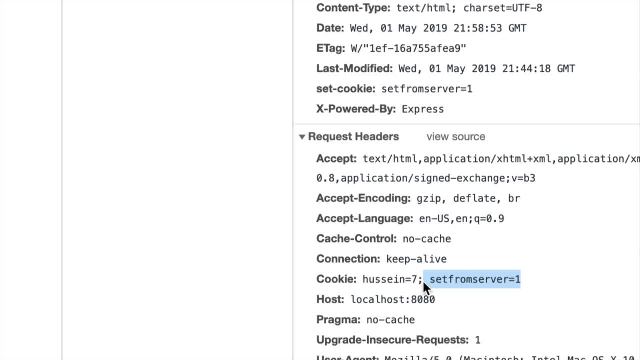 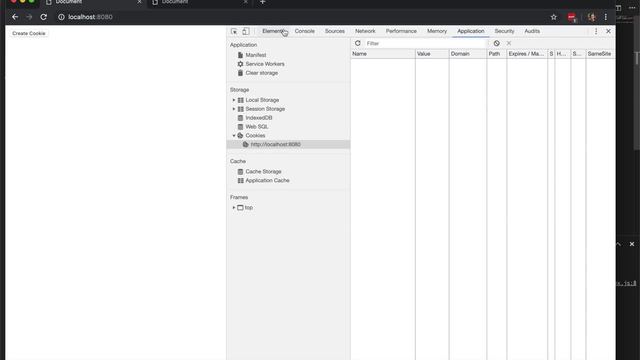 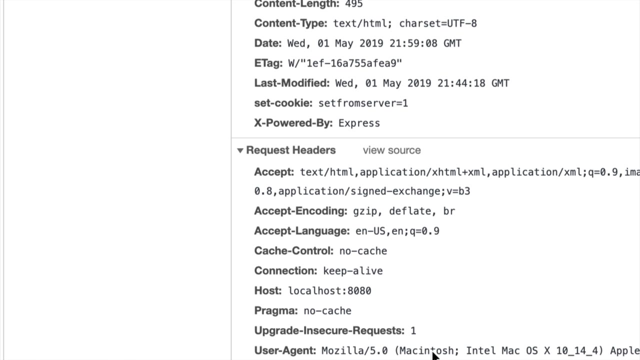 We, We have the old cookie from here and this is the server cookie that we have sent right. So the moment I clear the cookies and then I made the request again. right, You can see that I don't have any cookies. 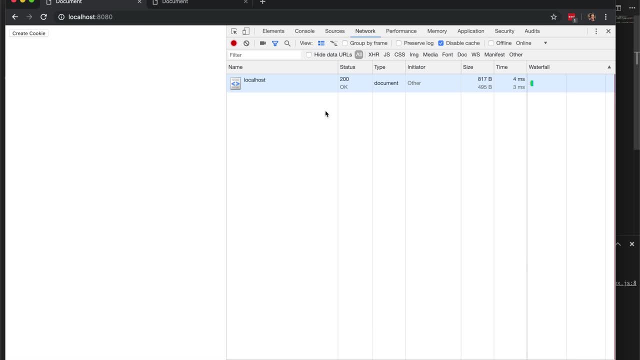 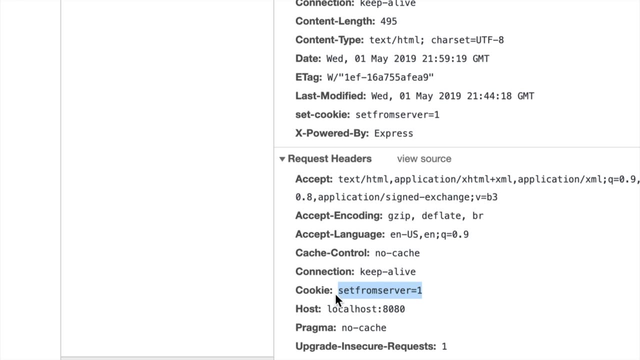 No, nothing got sent. The moment I refresh again, guess what One cookie is getting sent. You know why, guys right, The first week We cleared the cookies. Here's what we did here. Here's what we did. We cleared the cookies, right. 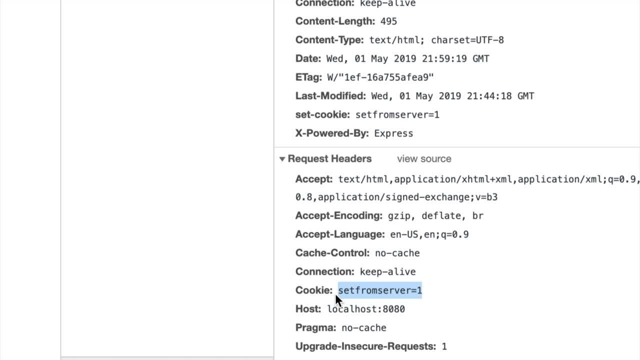 We. so we now we made the request with no cookies at all, right, So we didn't. we didn't send any cookies. The server told us: Hey, by the way, you don't have cookie, Please create. set from server cookie. 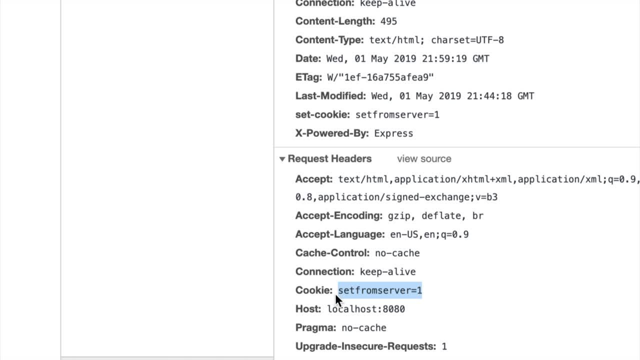 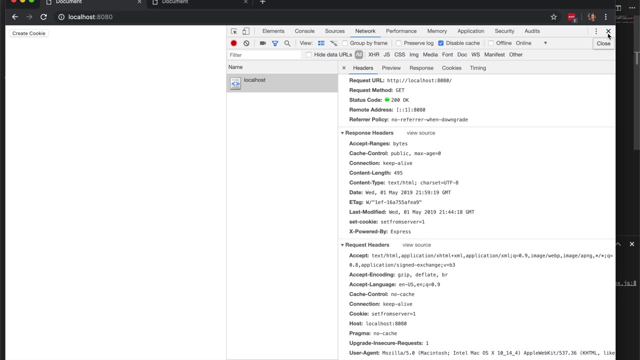 That's the server side cookie created the second refresh that we made, We sent that cookie, All right, And uh, here is so. So that's why we have the set from server cookie. All right, let's talk about paths, guys. 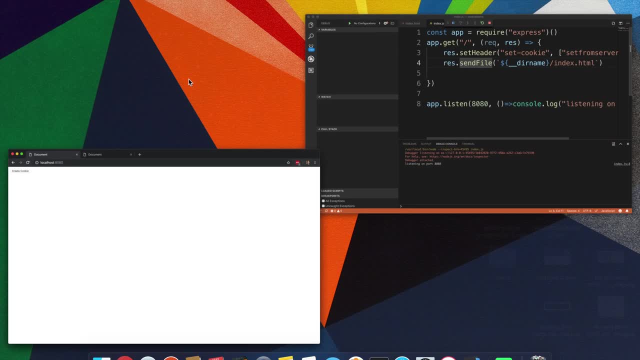 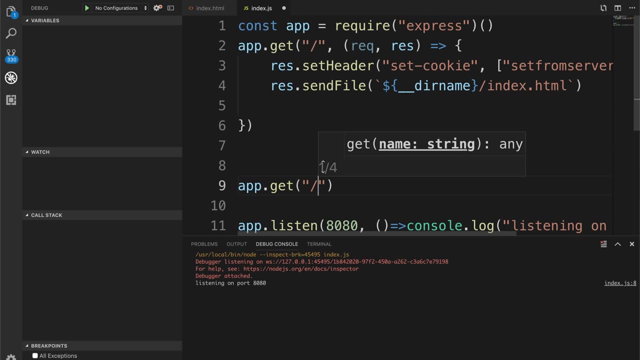 Let's do path now. All right, So path. I'm going to configure my application here with paths here. So I'm going to create a path. Yeah, let's go to path. one request response And what? what I want to do here is guys. 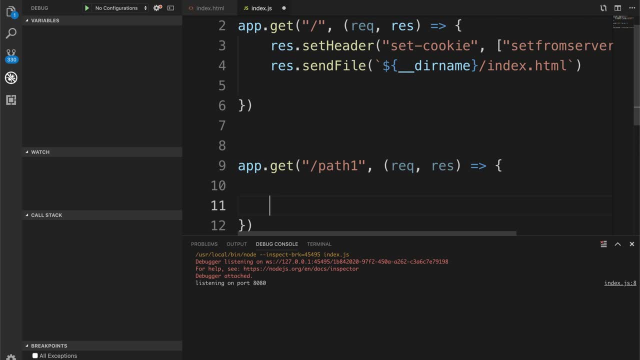 Literally When you make a request to the path one, I want to return the cookies that have been sent to me. Okay, So that's what I want to do. So, to do that we just like, literally, response to send, And uh, there is the. the cookies are part of the request. 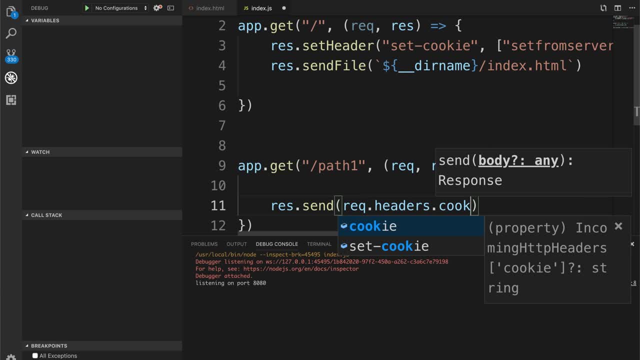 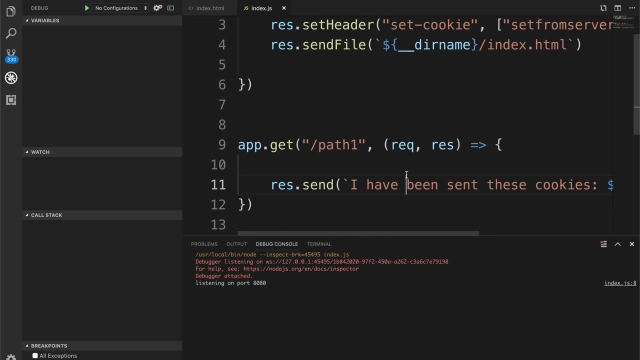 So request dot- uh, I think headers the cookie. there you go, Okay, And we can just do that. I have been sent these cookies, All right, so the server will just respond with the cookies that has been sent to. 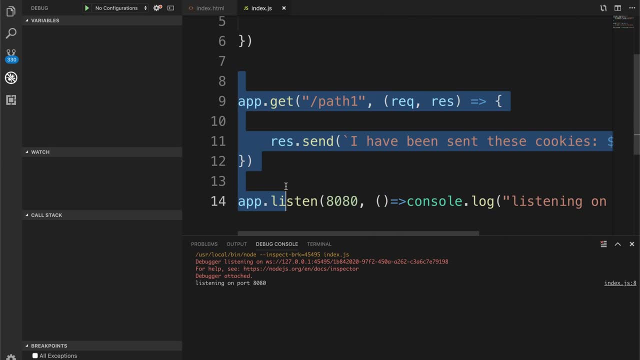 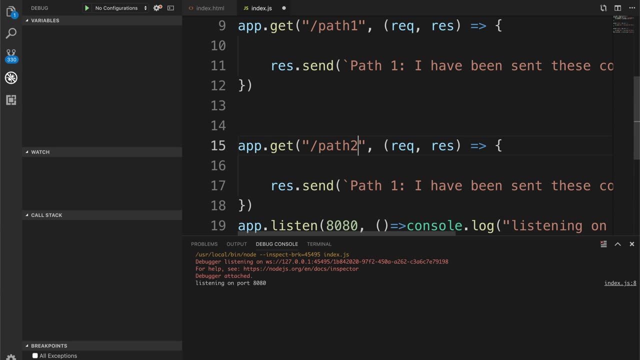 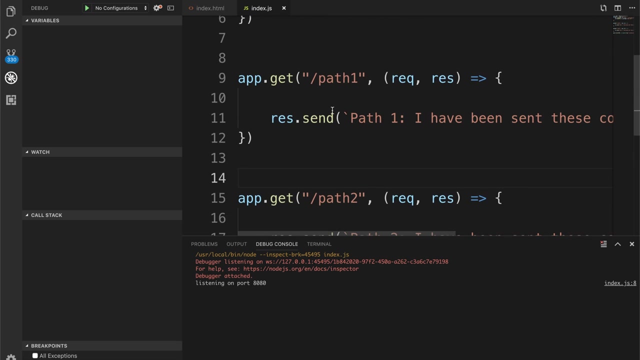 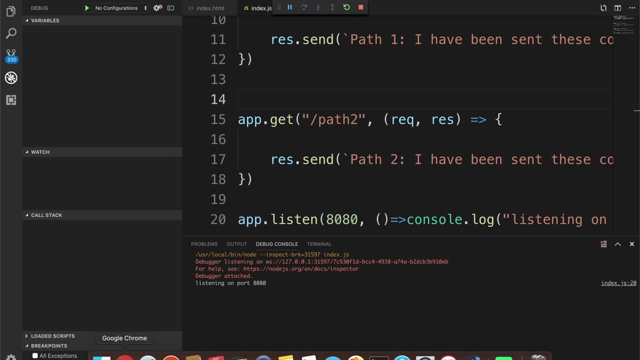 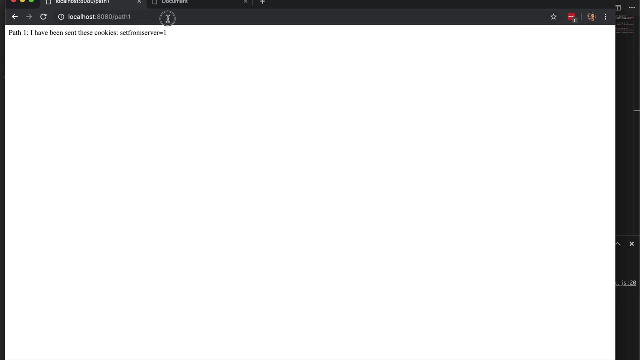 Okay, Okay And uh, let's just say path one, And I'm going to do the same thing, Path two. And here you go, Sweet, Sweet, All right guys. So let's do this, run Localhost, do all one. uh, that, do path one, we can do that. 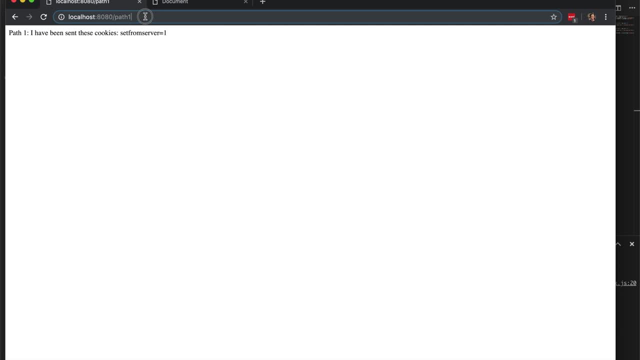 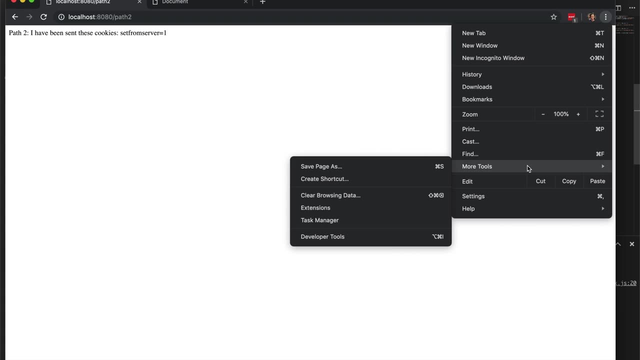 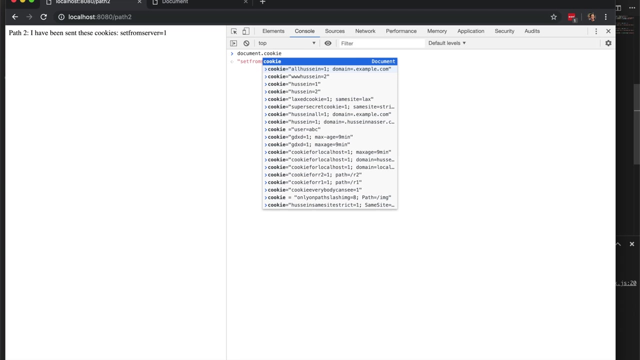 We can see that there's sit from server, which is that the default cookie that we got right. We do path two. That's the only cookie we have. Here's what we were going to do here. I'm going to create two cookies. document the cookie equal. 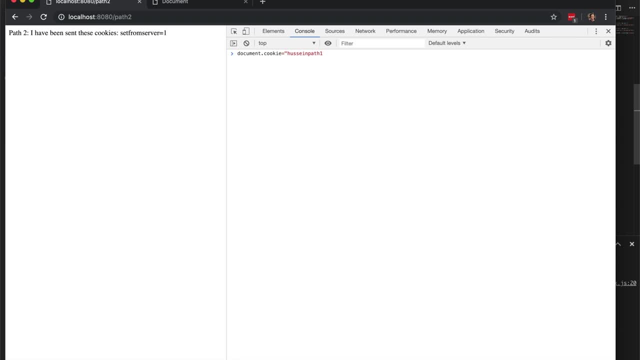 Let's say: uh, I was saying path one. I'm going to create a cookie that is will only be sent to path one. And here's how we do it. You add a property, Remember the domain. this is another property called path, and you can literally just say: slash path one. 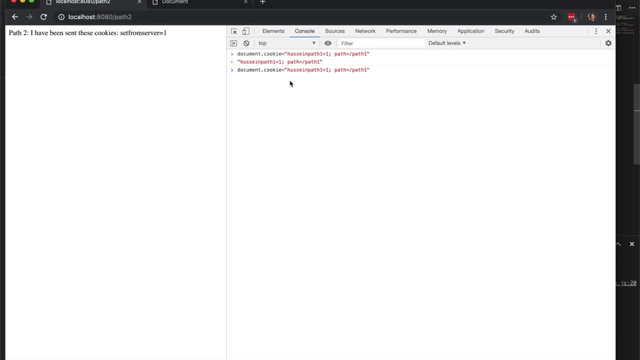 Okay, That's the first cookie. The second cookie is literally, I'm going to call it path two just for fun, And then just have another value. So just a completely different cookie. but it's only Okay, Set to path two. 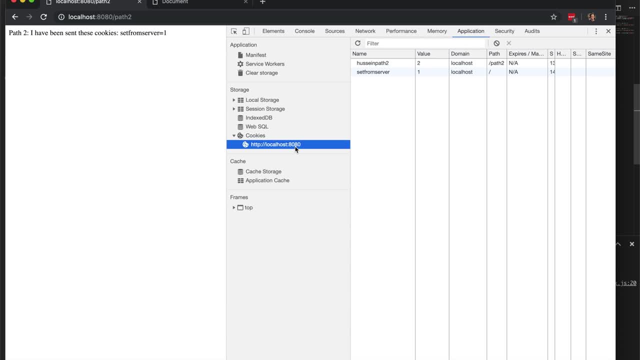 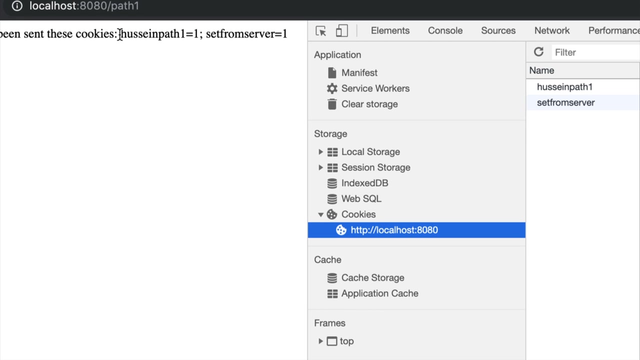 Let's talk a lot. Just take a look at the cookies here, guys, So you can see that. refresh, We have the same path too. Okay, And here's what we're going to do, guys. If I make a request to path one, you can see that the response came with the same path, one only. 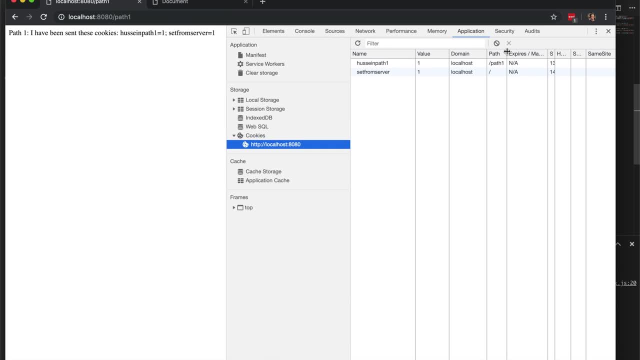 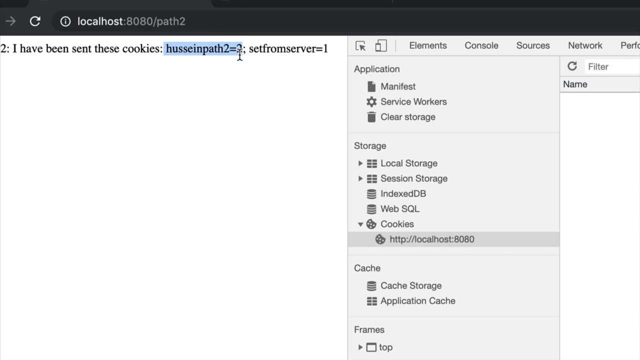 Right, And we can see that I can only see. this is what I can see. slash path one because I am in the path one, right. If I do path two, I get there is the other cookie right, But I also get this cookie all the time because this cookie has no path. 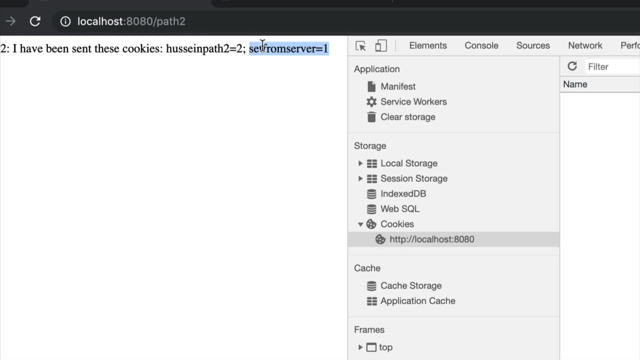 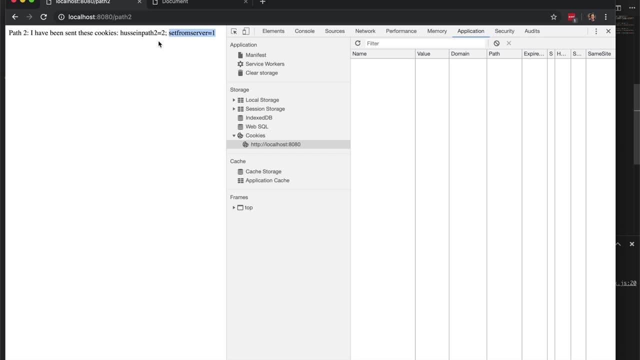 It is just like the path is universal: Always send this cookie to all path. So this is pretty cool, guys, Because now, if you have a huge set of cookies, you can configure them to be sent to only the relevant path, right? 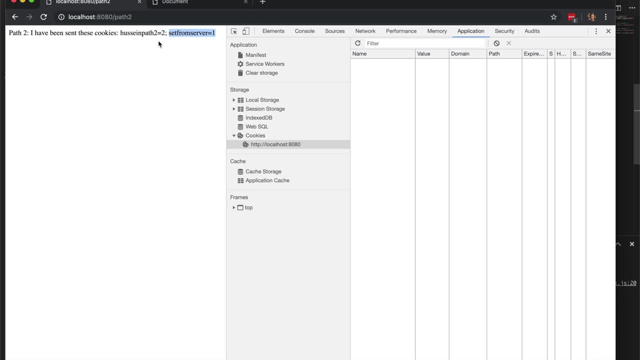 If you have that slash login or slash certain APIs, right. You don't need to send unnecessary cookies to the login API or the login path. if you're not going to use it, All right, And the reason is because you are going to save a lot of bandwidth, right. 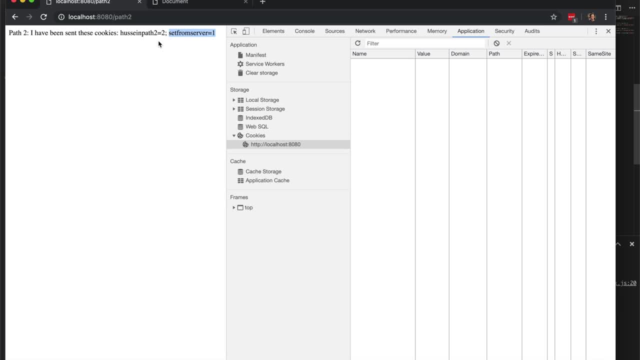 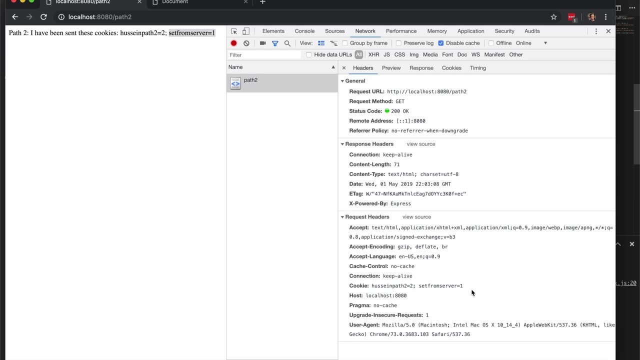 Because cookies are going to cost a lot of bandwidth, right? Because you're sending it with every request. They are kind of stuck with you And we're talking about small cookies here, But in real life you're going to have a lot of cookies, a lot of strength and big name, big big bites, right? 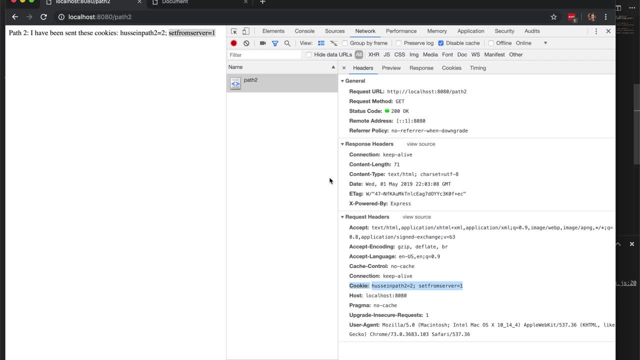 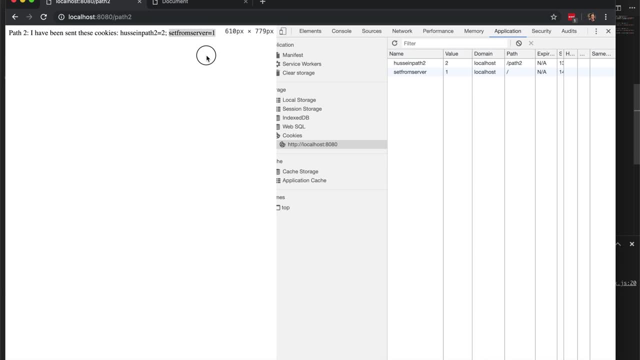 Especially with sessions. So you need to be careful with that right. So use that right When you feel it It's worth it, right. But path is good Path. This is the path. This is how you do path right. 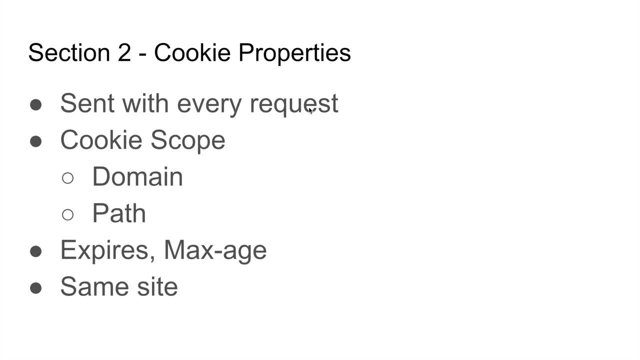 So, all right, Let's go back. What do we learn? We learn about sent. with every request, We learned that cookies has scope, domains right And path right. I can send certain cookies to certain path. I can send the domain, the cookies for a certain domain. 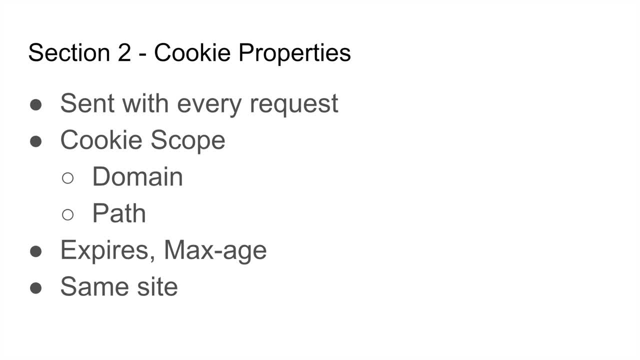 All right, Expires and makes Age kind of kind of the same guys. but cookies, if you don't specify these properties- expires or max age- the cookie will be destroys. destroys the cookie. who will be destroyed when the browser just closes right? 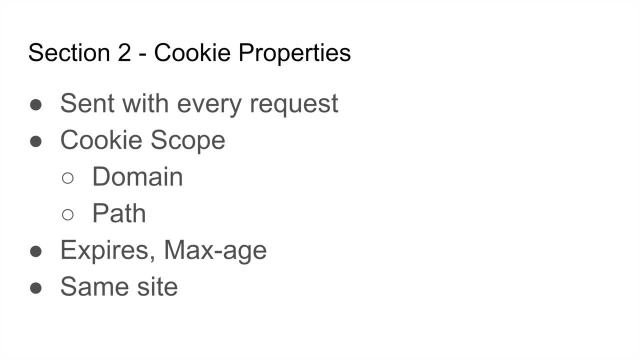 That and that's called what we call the session cookie right, Which will come to it right? If you don't specify a max age right, Then the cookie will always get Destroyed If you close the browser. I'm not going to demonstrate that. 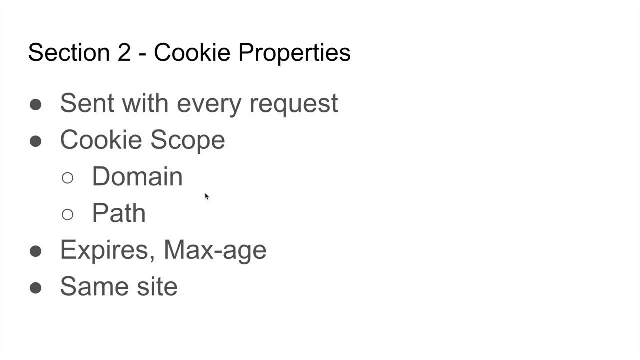 I think that's, that's just it's. I mean, maybe we'll, we'll show it right. But you can say: max age equal three minutes and then or the cookie. if you do that, then it's called the permanent cookie, which is kind of weird name because it's not really permanent, right? 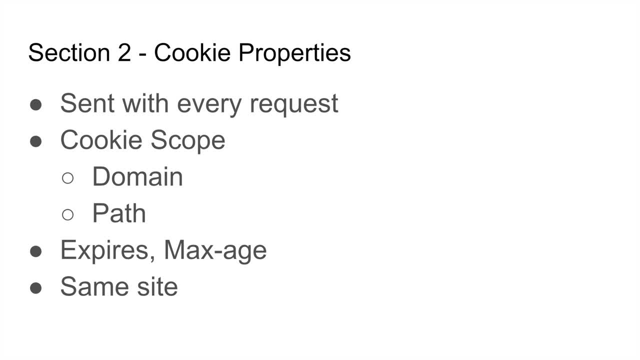 But it's called permanent for some reason. that the MDN calls it All right. So if you set a max age or expires, is good, it's called a permanent cookie, right. What do we get? I do is, uh, essentially it has a lifetime. 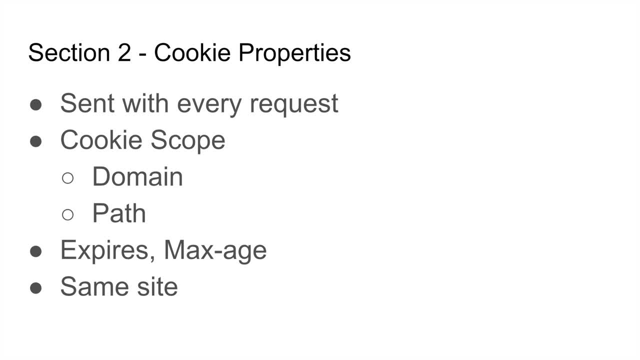 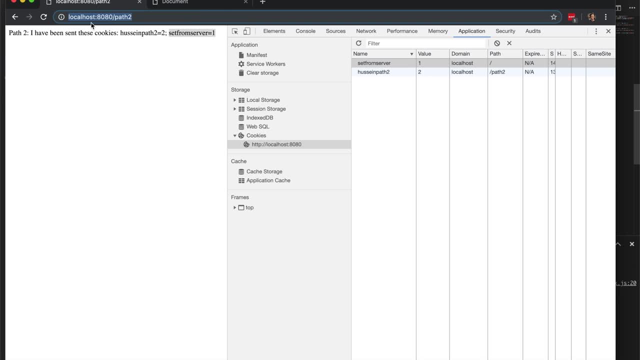 Even if you close the browser, it still lives. If you open a browser again, it still lives, right? So yeah, you know what, guys? let's show you a demo, because I am, I am that cool guys, Okay. 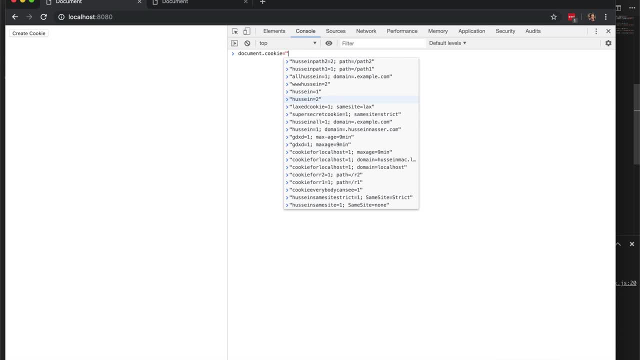 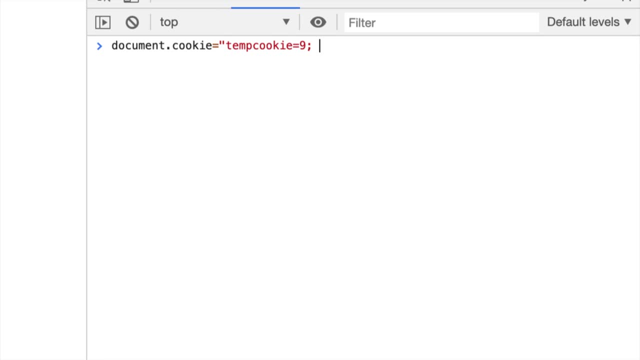 So I'm going to create a cookie, Let's say temp cookie, And this cookie, Well nine, That has max age equal, I don't know, three minutes, Is that? is that how you do it? I don't even know. 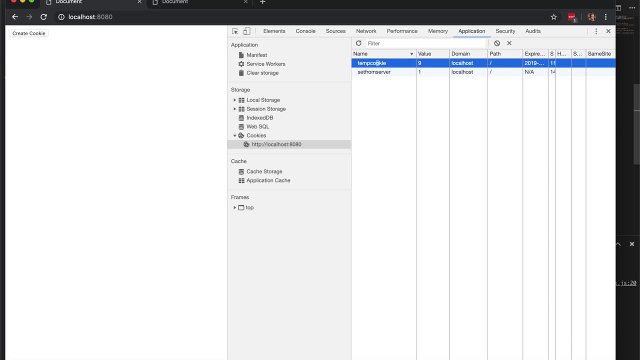 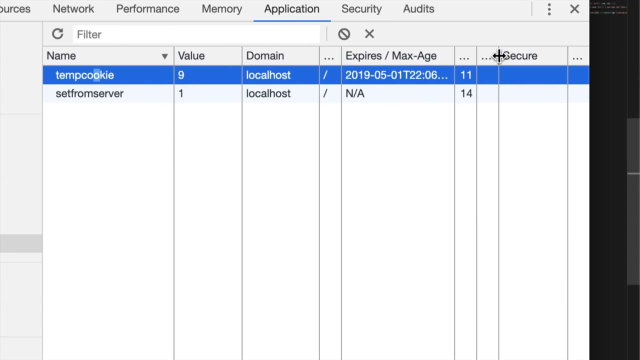 Hopefully that that does the trick. There you go. That did the trick, guys. If only I can expand this. there you go. So this will expire after three minutes, which is literally that's the date of this thingy. So it's going to expire on. 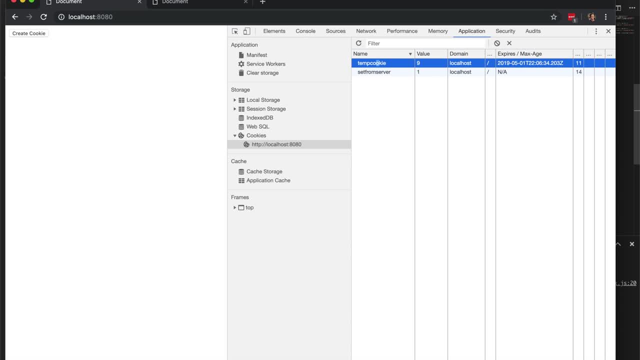 Whatever this day- it is May 1st- All right, So it's going to expire after three minutes, right? So that's that's how you do it. If you don't specify, it's going to say in a, which means not available. The moment you close the browser is just goes away, Right. But Chrome doesn't have. has this weird thing with- even with session cookies, right. Even if you close it and do specify a max age, it comes sometimes, it just keeps them. 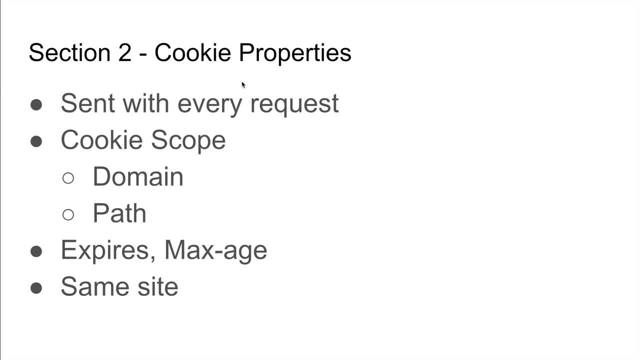 Right, I don't know why, but that's, that's Just. you can't take my word for it. Okay, Expires max age. So you, you, you need to set them If you need to keep your cookie alive for a while. same side. 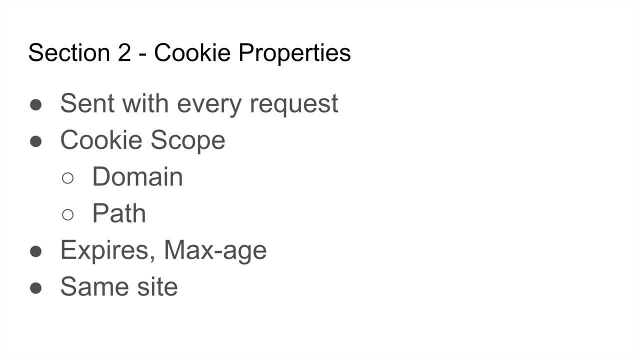 All right, This is my favorite Right. It took me a while to understand this, to be honest, guys, It's it's a kind of complex thing, Right, But once you understand, it's a really basic, simple right. 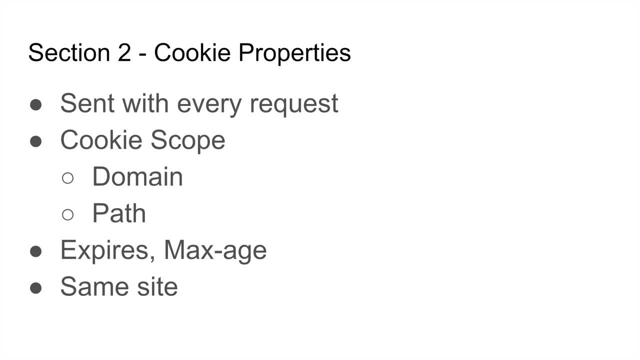 But that that makes me really think. it's like, wow, I don't understand anything about these cookies, Right. And then, and it's pretty cool Once you do understand it, Right, And that was it's good guys to have this mindset. 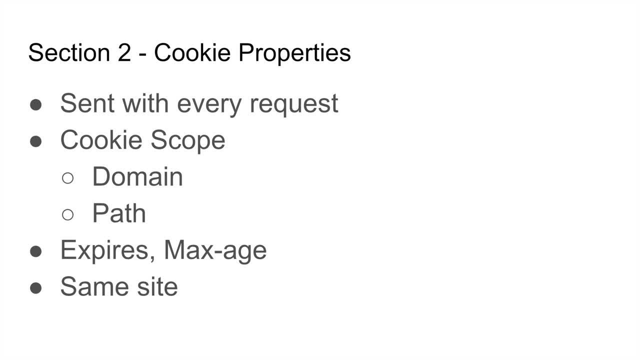 It's good to have this attitude of about everything in life. really, It's just like treat everything that you don't know anything. If you treat every, if you treat life that you you know everything, then you kind of don't will not learn anything. 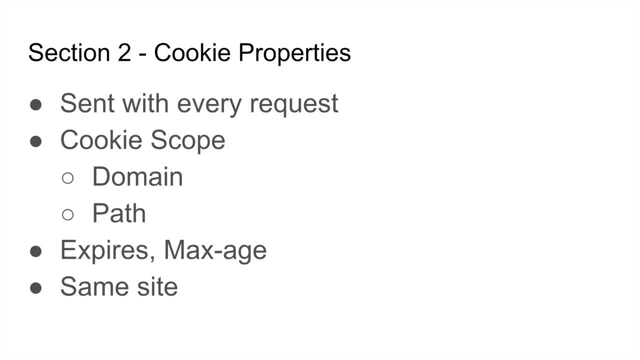 Because you you'll always be arrogant and you'll always like think yourself like above others, Right. But if you treat that, everything is like a new opportunity To learn, right, All is accepted. It's pretty cool How much you can learn. 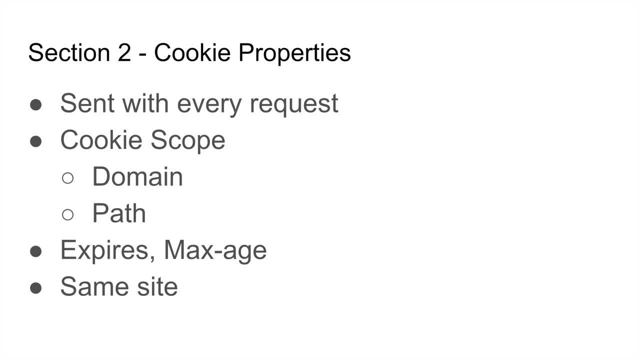 All right, Sorry for the life lesson there, guys, but let's do that. All right. Same site, Same site. This is. this is. this is really new, I think it's like. I don't know when it was added, but it was recently added. 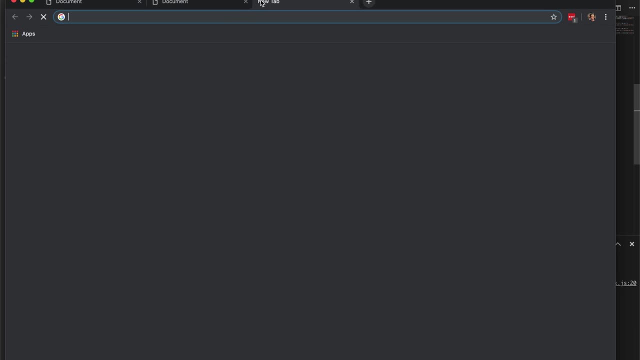 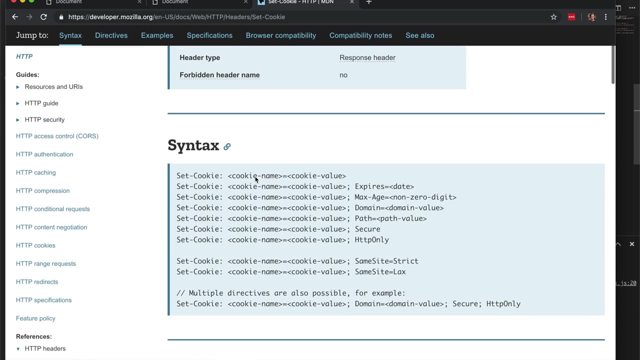 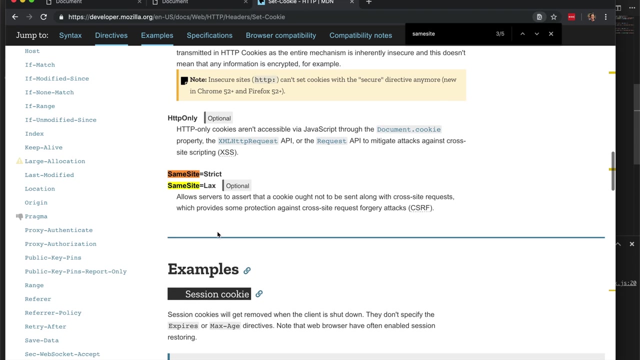 And I think Chrome added it first. I don't know if it supports You know what. Let's just let's actually check Same site: MDN. Same site. Yeah, So I don't know when it was added. Yes, 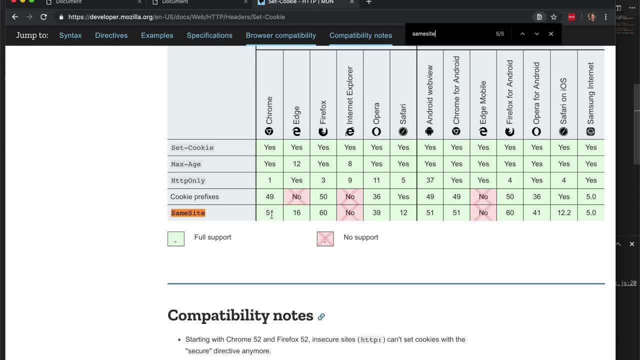 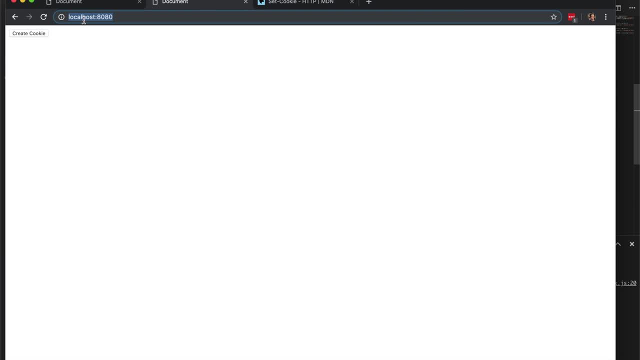 It's available in all browsers, But I think Chrome is the first one that added it. All right, So let's explain what this thing is, guys. All right, So here's here's. here's the problem, guys. Okay, Let's assume. 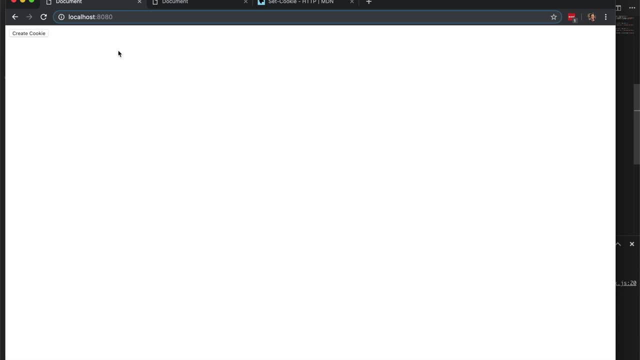 So you, you logged into Bank of America, Okay, You as you logged into Bank of America, Okay, And Bank of America uses the set cookie header and they set your session ID and a bunch of other stuff- tokens and all that stuff- in your cookie. 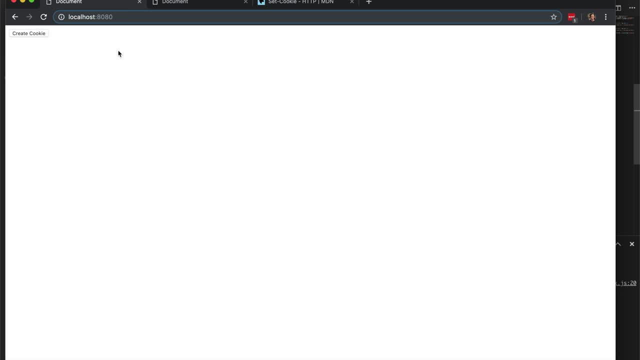 So now your cookie has these tokens. So now you, when you go to bankofamericacom, you don't have to log in because the cookie is always sent with each request. So the server says, Hey, Oh, it's you. 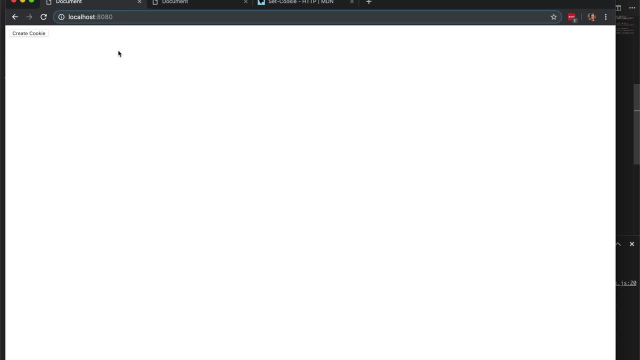 It's. it's Barbara, So I'm going to log in Barbara, Right? I don't have to ask her for credentials. Okay, Right. So that's how you do it. You literally go bankofamericacom and enter. 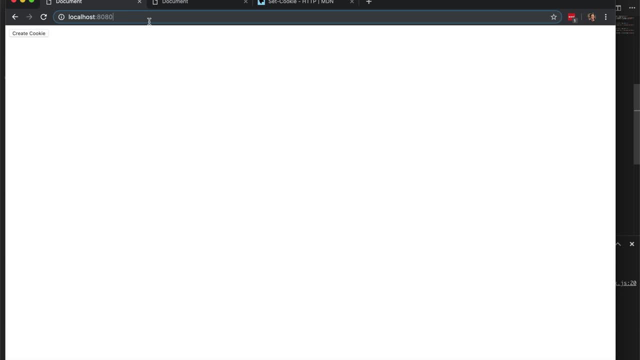 And that makes the browser have your cookies and we'll send it with every request. We talked about this, right, That's, that's the basic thing. All right, Now imagine this scenario. So there is one way to do anything: going to their browser and typing bank of America, right? 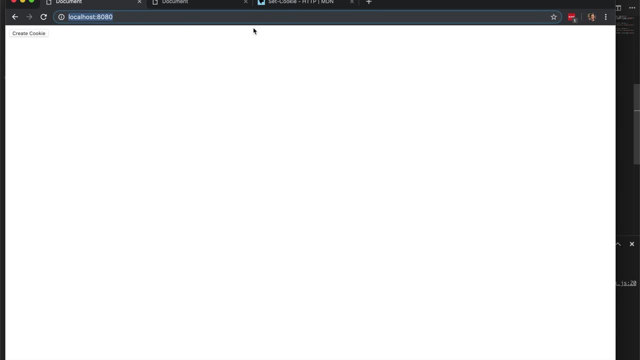 Or the browser or the site examplecom or anything, right, And you hit enter yourself. There is another way of what? if I have a link here that goes to bank of America, right? If I have a link, literally just click here to visit bank of America. 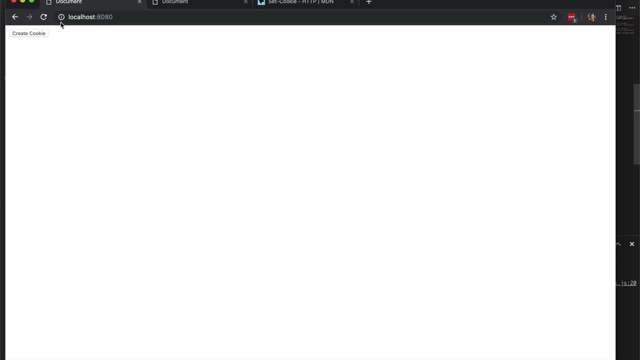 I am on, I don't know, The pirate bayorg, Okay, And then I click on that link that takes me to bank of America, the browser. guess what? will the browser send my cookies to bank of America? The question is yes, it will send it, which is kind of freaky, guys. 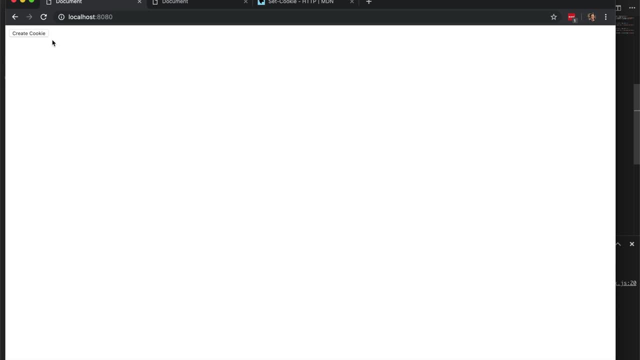 If you think about it, if you're in a just shady side and this side has a link and you click on the link. That's why people, People tell you don't click links. It is really scary, guys, because if you have cookies, like from your bank or whatever, and you click that link right. 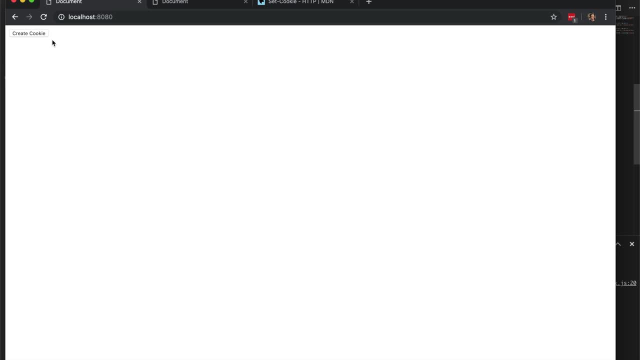 The broth. Remember that that site doesn't have access to your cookie. It will never have access to your cookie, but it will make you click that link which will Will take you to that Site with your cookies. So it can do bad thing just like that. 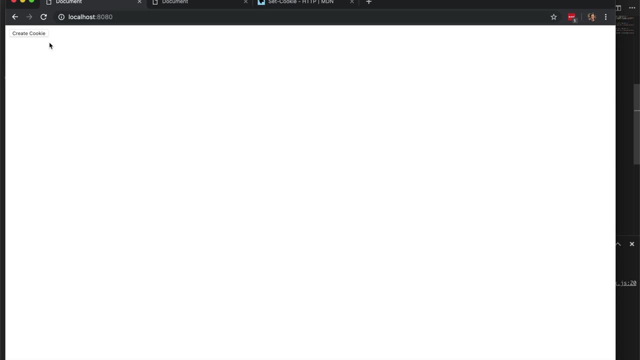 We're going to talk about out. But yeah, if you have a link, you're going to send that cookie, right? All right, So let's give me, let me, let me give you an example here. Okay, guys, So if I have a link here, 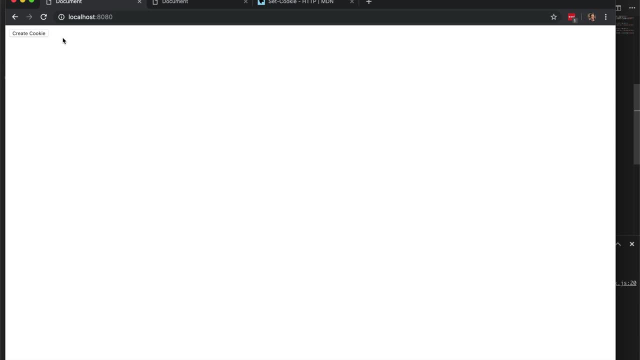 All right, Uh, if I have added a link here and I add, uh, I'll ask you to click on this Right, And this link has, let's say, uh, it goes to bank of America, but it doesn't go to bank of America. 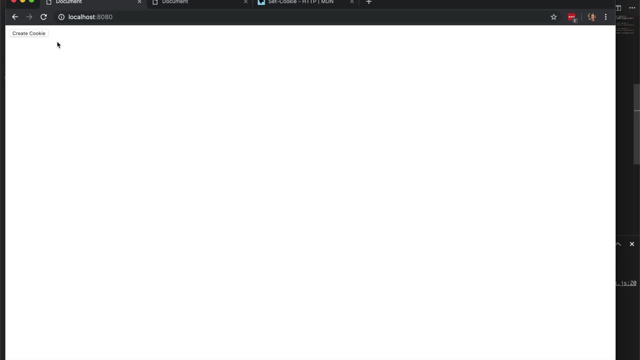 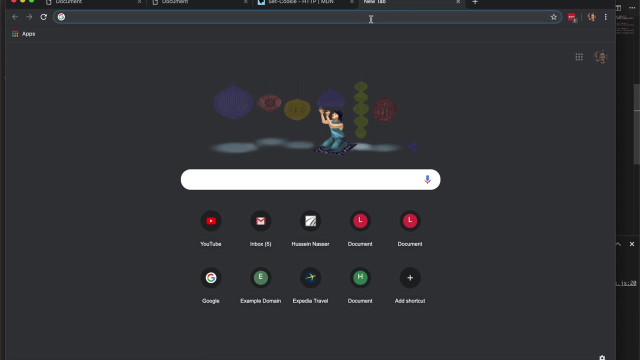 It goes to bank of americacom slash. Let's say these guys are lazy and wrote an API called slash transfer money And there is like an and percentage. All right, Let's actually show you about that B of a bank of americacom slash. 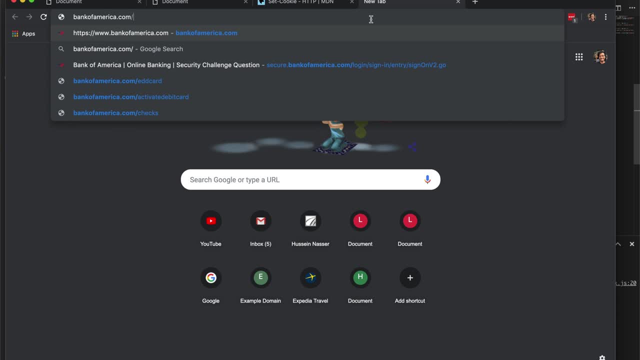 That's actually my site. now I'm not going to go there, Don't worry guys. But let's say there is, there is like a, there is like a. But let's say there is, there is like a, an API called transfer. 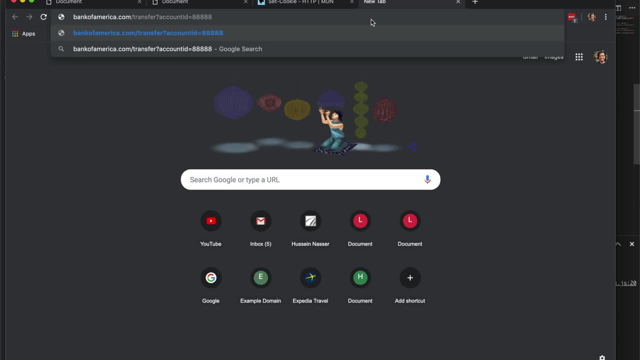 And there is an account ID equal blah blah blah, And then let's like, a money is equal 1 million, Right, Let's say, if this actually transfers 1 million, What's this 1 million? What is this? 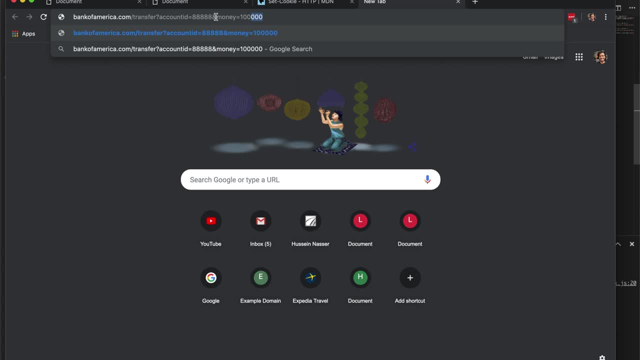 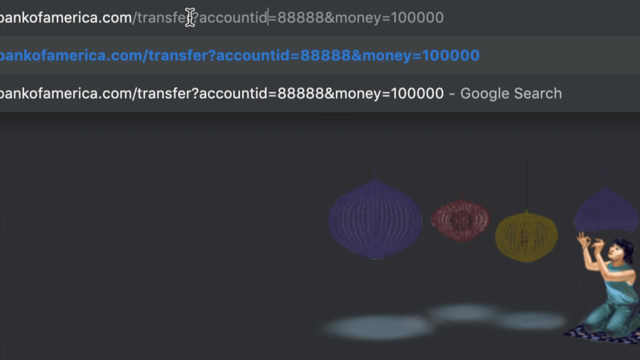 That's a hundred thousand, A hundred thousand dollars from your account to account 8888.. That's what it does, Right? That's the request. It does that, Right. It transfers the account from your session, Right, Because this is the two account. 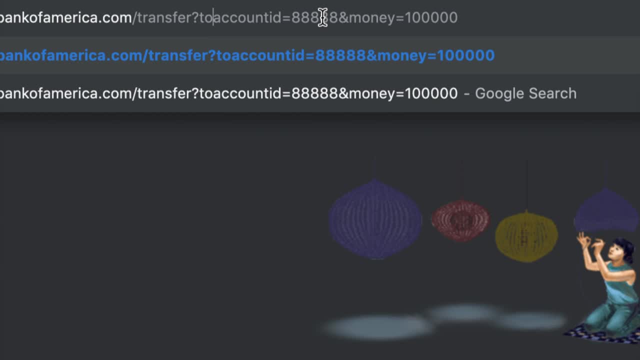 Right, This is the two account ID. Okay, But you are already logged in, Right, So it will transfer your account from your account, Right? But if you, if you are not logged in, this will fail. If you're logged in, this will succeed. 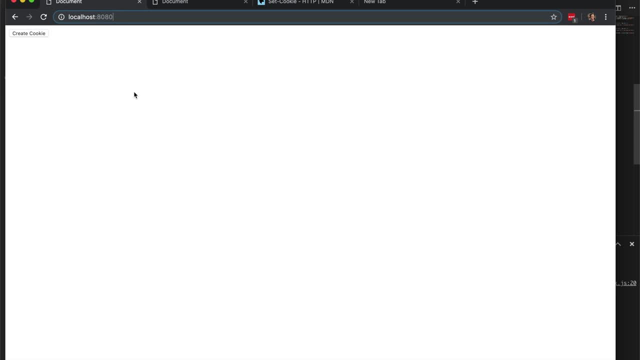 So if someone have this URL on a shady side and you clicked on it, they will, for they will, like, kind of, force your account. They will force your request, forge your request Right To transfer money from your account to their account by one click. 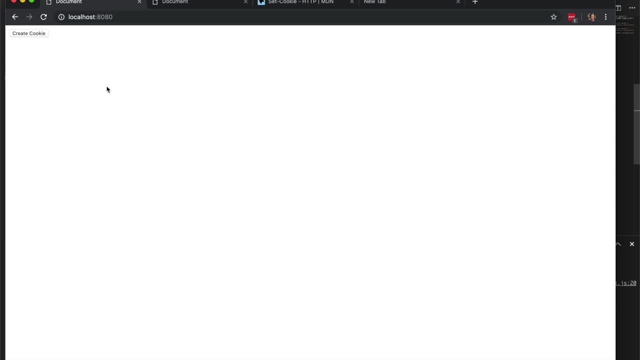 All right, And other bad things can happen as well. Okay, If that's a fifth, it's a link. If it's kind of it's a post or a gate request using fetch, then course will take care of that, Right. 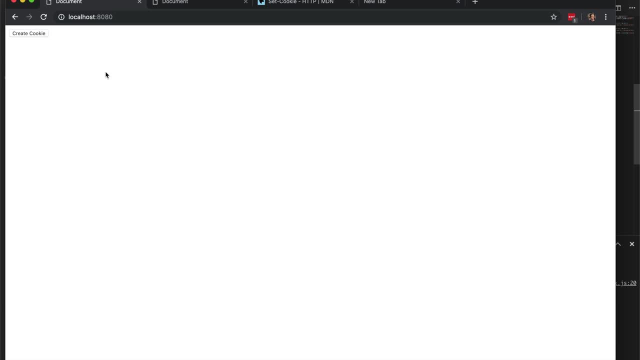 Yeah, That cross origin resource sharing, which we made a whole video about it and you guys loved it, Right? I'm going to reference that video here, Hopefully, Okay. So so if you make a request here and you make that request to bank of America, you. 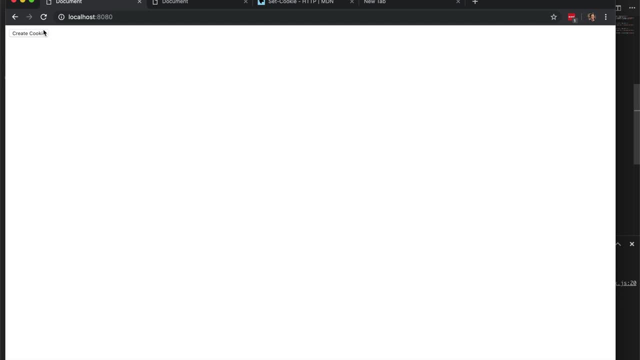 can. you will be blocked because bank of America says: Ooh, wait a minute, you are a shady side. You cannot make a request to me, Right? You're going to make a post request. You can make a get request. 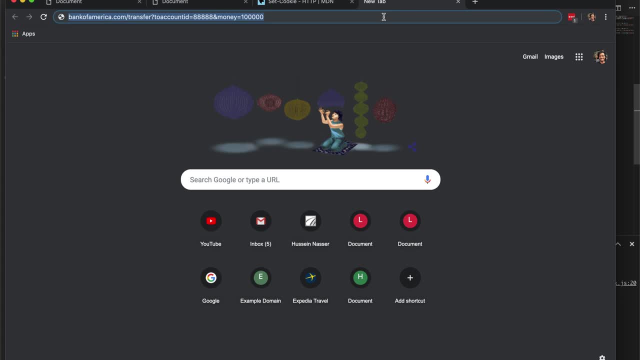 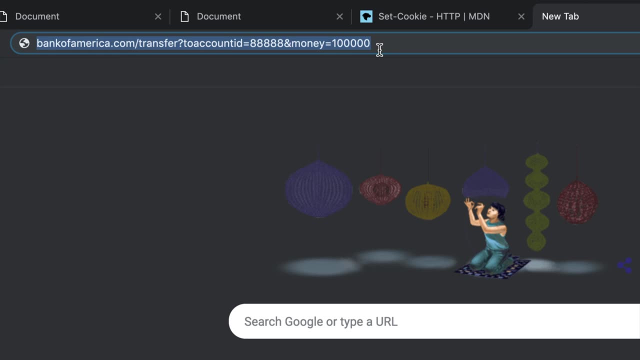 Right. So we got that. that, uh, that this, this, this example is kind of- uh, it's kind of what was the word for it? It's, it's contrived, guys, because this, when you do this record and you hit enter it's. 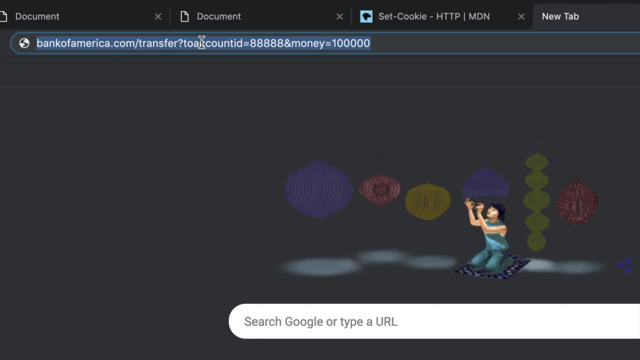 actually a gate request and nobody in their right mind will make a transfer uh API as a get request. That's the most insecure thing in the world. Plus, banks now have all this capture. That's why banks suck guys Dealing with banks. 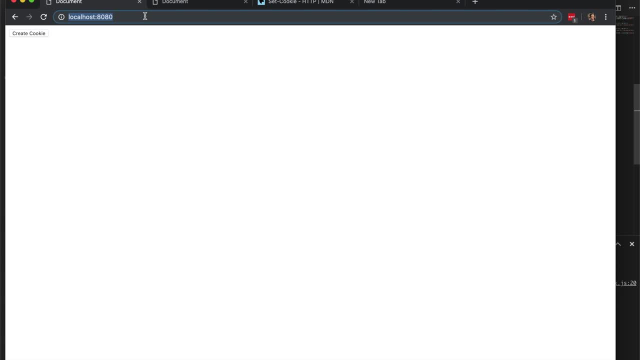 Like: do transfers anymore. You transfer some money, You have all to do, all these captures and captures and all that million notification. They have to send you a message to their phone just to make sure that it is you right, Because they don't trust anything. 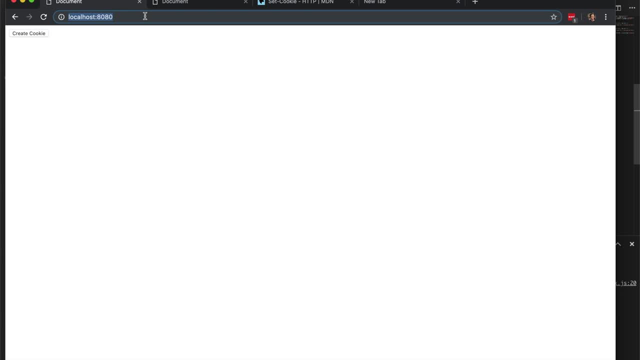 Right, And that's a good thing, Right, That's what user experience with banks suck because of this, because of the security. Okay, All right, guys, let's show you how this works. Some same site, All right, Sorry for that long grant there. 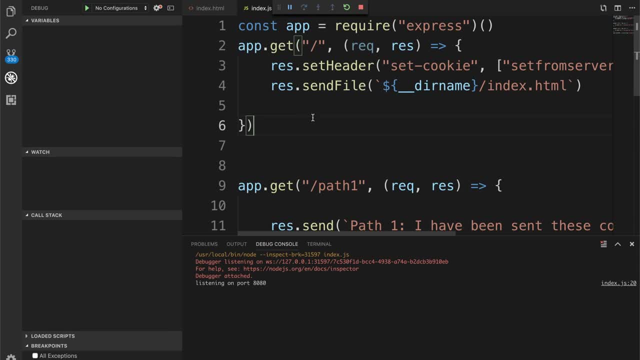 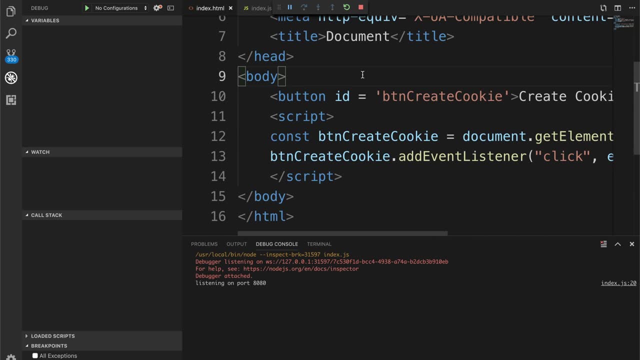 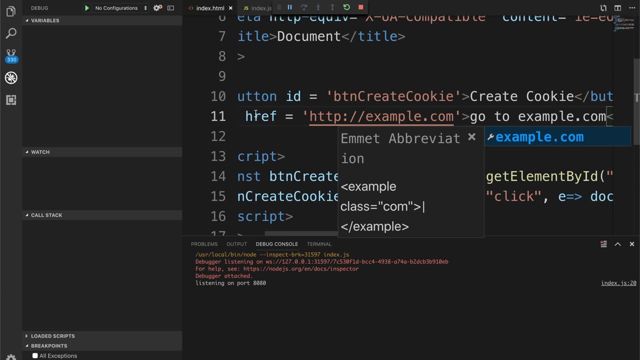 Um, all right. So we talked about path. What are we going to do? Okay, Go to industry html. I'm going to add a link and here's what I'm going to do: a href equal. I'm going to do examplecom. go to examplecom is right, guys. 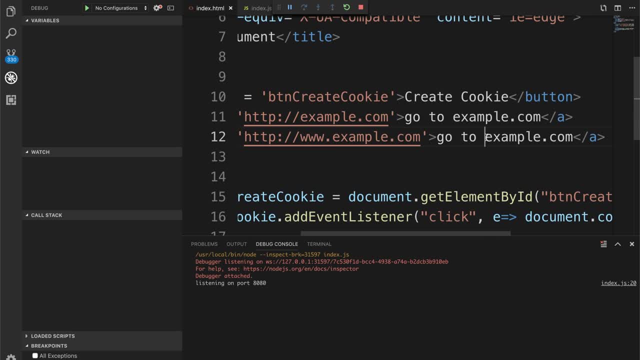 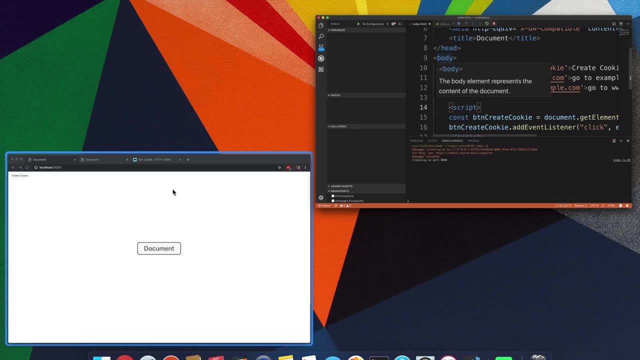 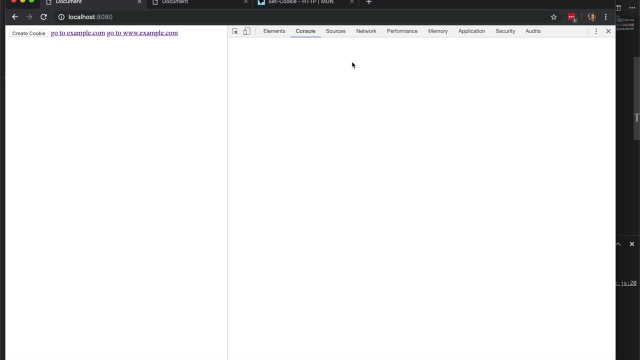 And this is go to wwwexamplecom. Remember those two guys, right? These are. those two have different cookies, So let's see what will happen by refresh. Now, if I click this, let's see what cookies will get sent, right. 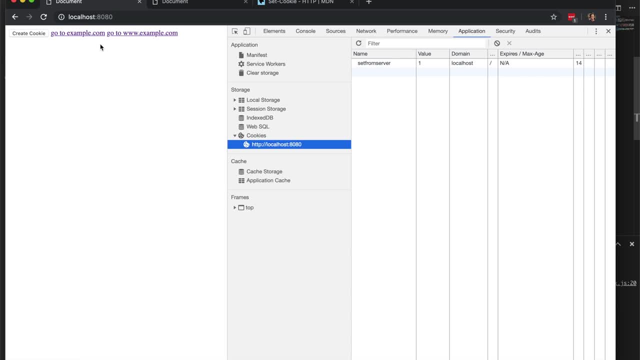 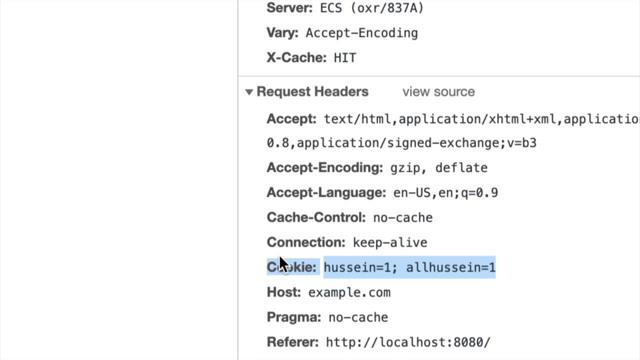 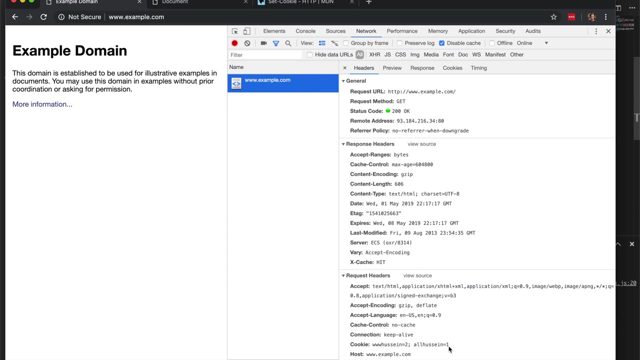 If I go to application, right, If I go to examplecom, look what we sent. We sent Hussain equal one and all Hussain equal one. We send those cookies, All right. And if I go to This guy, we sent those cookies. 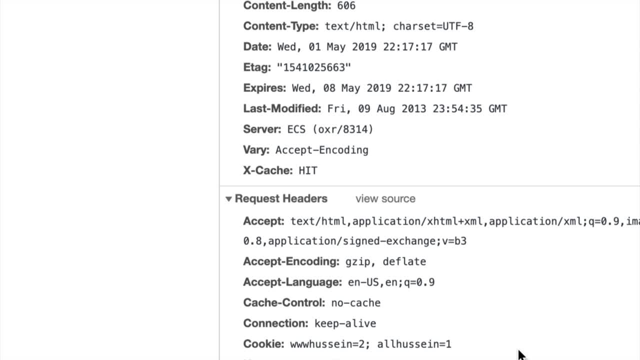 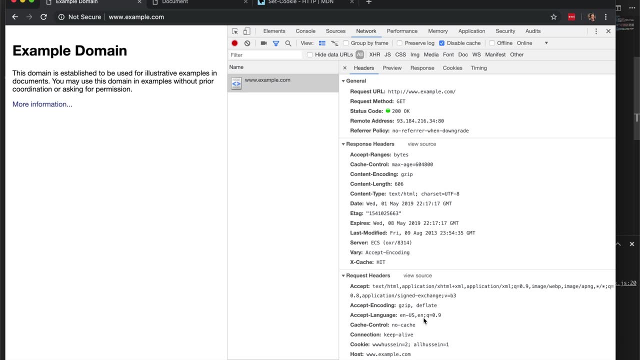 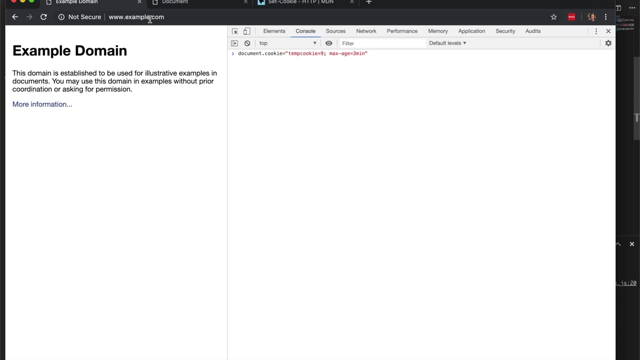 So we're sending cookies from that site. Okay, We're sending all this information, even if I am in a in a different site. Okay, So here's what are we going to do, guys. What I'm going to do here is I am going to go to wwwexamplecom, right. 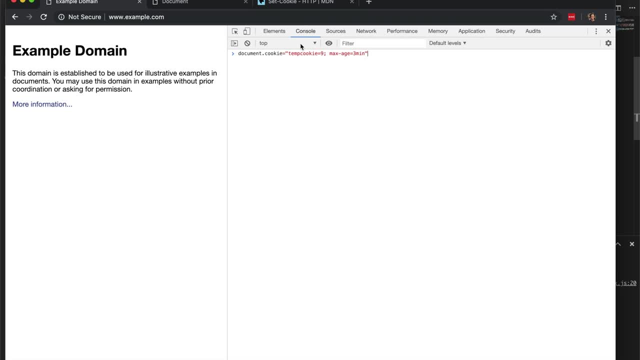 And, uh, let's, let's first. uh, let's see. Okay, Okay. Okay, Let's keep those cookies. All right, But I'm going to create a brand new cookie here on wwwexamplecom, but I'm going to. 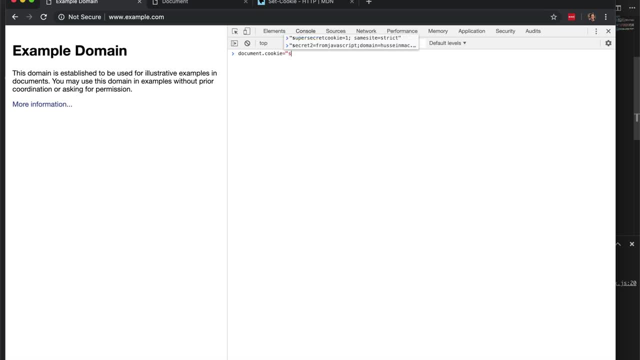 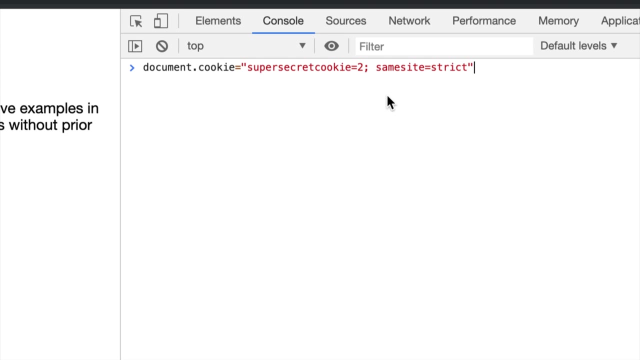 call it super secret cookie. All right, Equal one. And I'm going to add a property to it called same site equals strict. If you do a same site equals strict, then you will never get the same site. Okay, Okay, So you will never get this cookie unless you are in the same site. 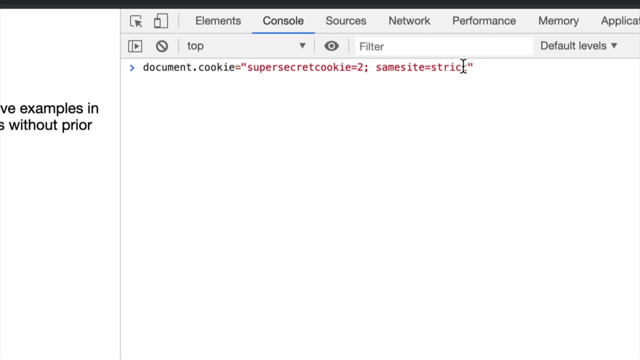 If you're in the same site, then the cookie will be sent to the server. If you are not in the same site, it will never be sent to the server. Okay, Makes sense, guys. So let's do this cookie. We just set a cookie called super secret cookie two. 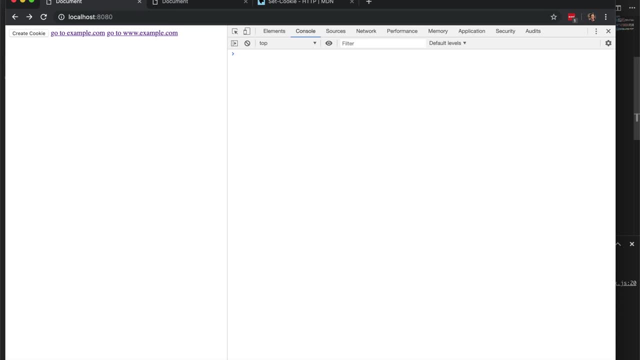 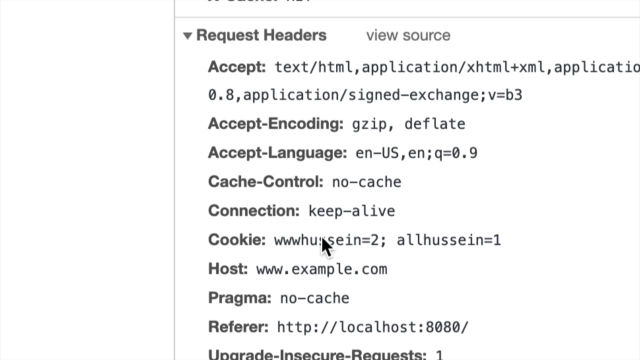 Right. So now if I go back and refresh, go here, go to network, We can see that the the cookie will not be sent to the server. the cookie was not being sent right. But if I visit this like normal, let's say from here: 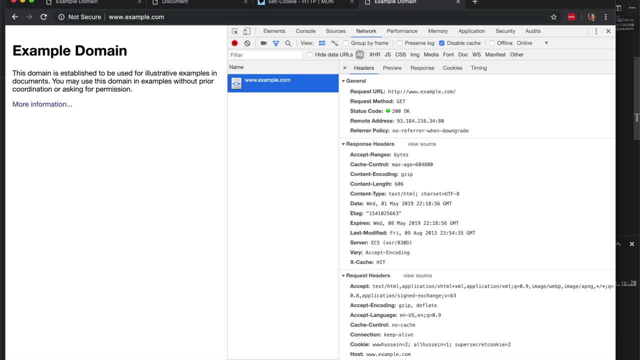 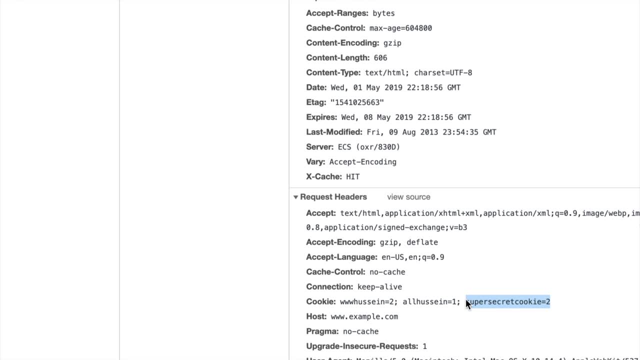 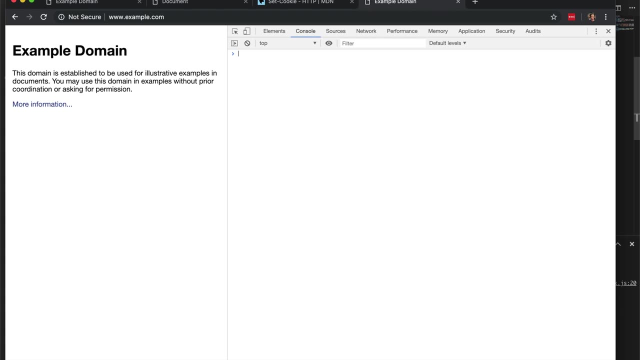 okay, wwwexamplecom, you can see that we got our super secret cookie. Isn't that pretty cool guys? So that's one way to do a same site cookie. That's the one way. The other way is to do document cookie. 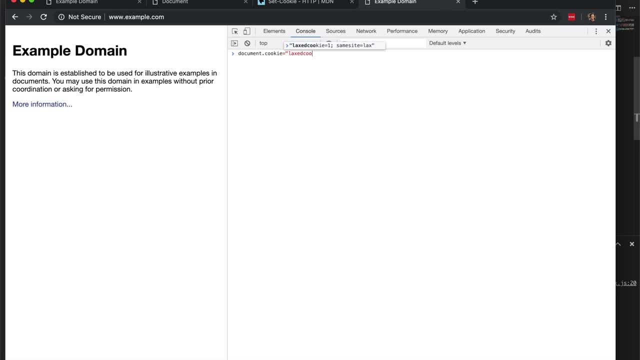 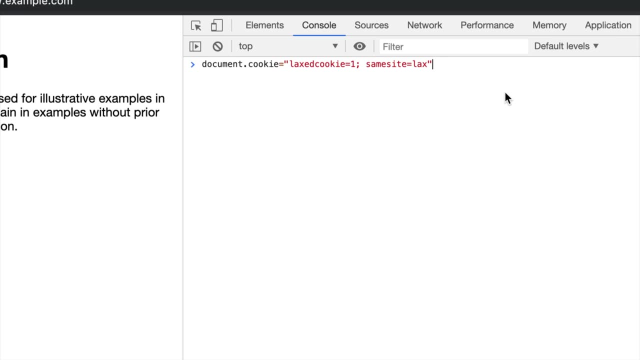 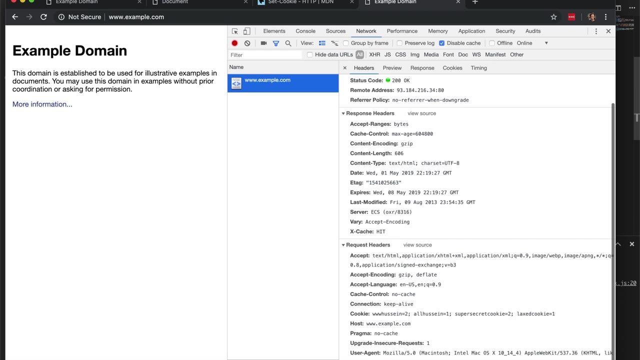 equal, kinda more laxed cookie, right. If you do another cookie same site, equal, lax, that's the other property- then that property, that cookie will be obviously sent. when you go to examplecom, right, Laxed cookie. But if you go to your fancy site, 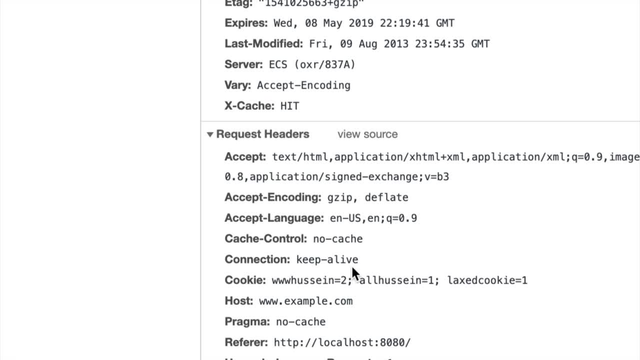 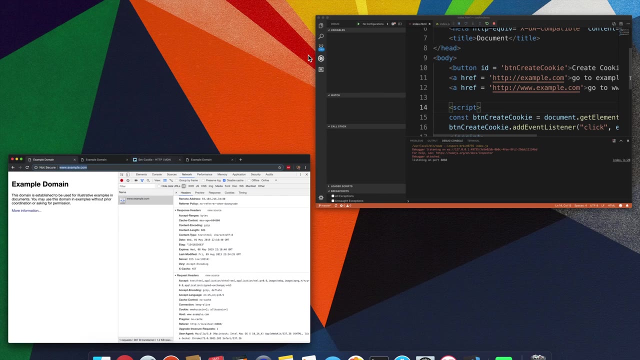 it will. the super secret cookie will not be sent, but the laxed cookie will be sent, because it doesn't. it's kinda more relaxed, right, It will be sent regardless. Makes sense, guys. So that's the same site property, right? 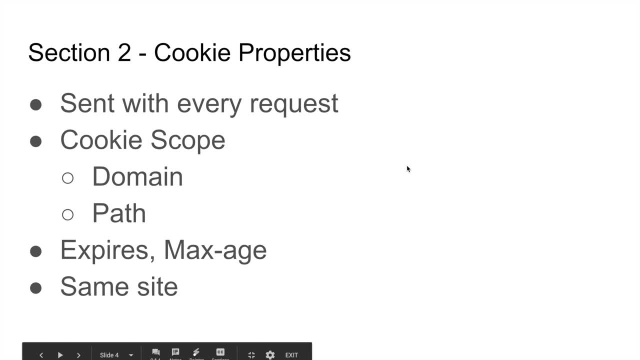 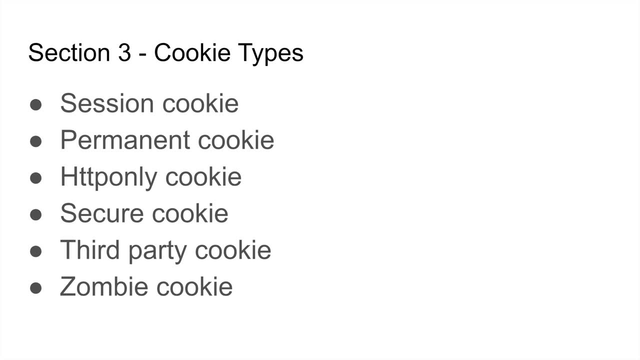 So we're done with the property. Section two is done. All right guys, All right, let's move on. What do we have next? All right guys. Section three: cookie tie, Cookie types. So take this with a grain of salt. 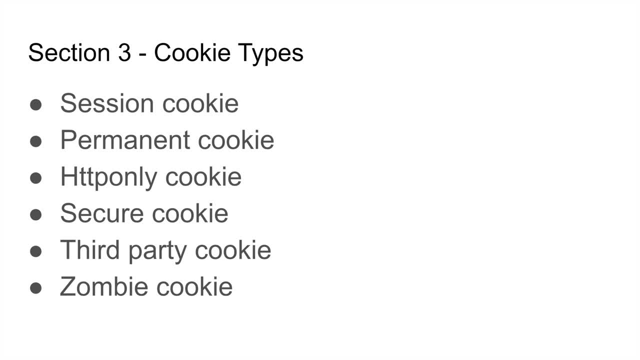 These are not written on stone cookie types, right? These are just the types that I've seen from researching this topic. Session cookie is the first one and we kinda talked about this. I'm not gonna demo this because we have seen this. 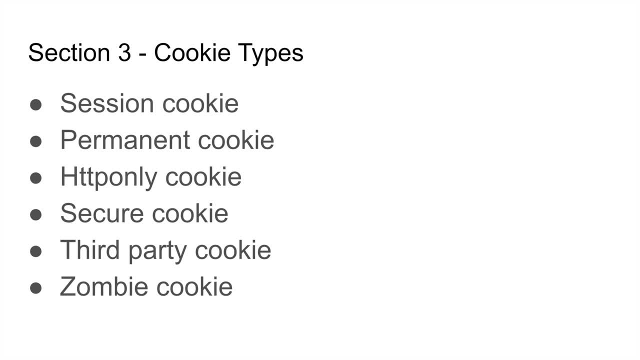 Session cookie is a cookie that doesn't have a max age or expiry. That means if you close your browser, your session ends and the browser deletes the cookie. right, That's what it means, Very simple. Permanent cookie is a cookie that has a max age set. 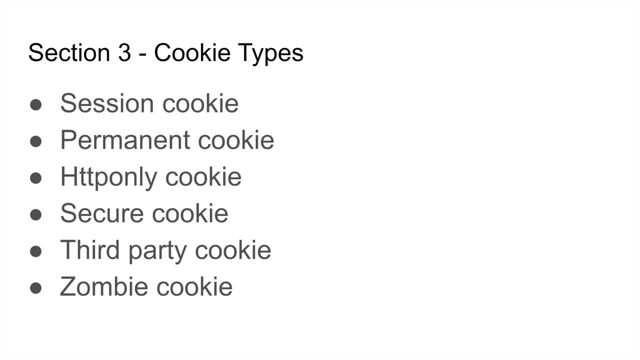 or expiry right, Which means once you set that expiry date right, It can live. if you close the browser, It can live after you restart your server, but obviously if you clear your cookies it won't live HTTP only. This is exciting stuff, guys. 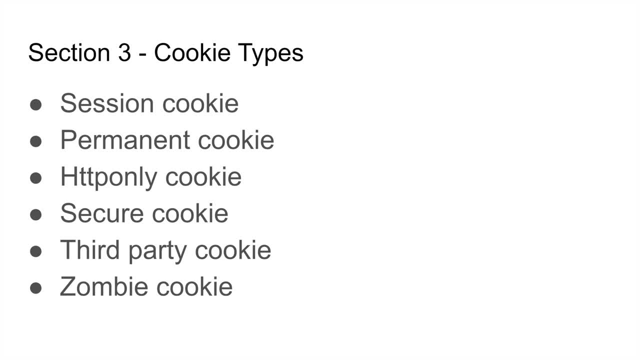 We're gonna talk about this now. HTTP only. cookies are cookies. guess what? That can only be set from the server and with this property, that's called HTTP only. And guess what? The browser cannot read them, and that's a security thing. 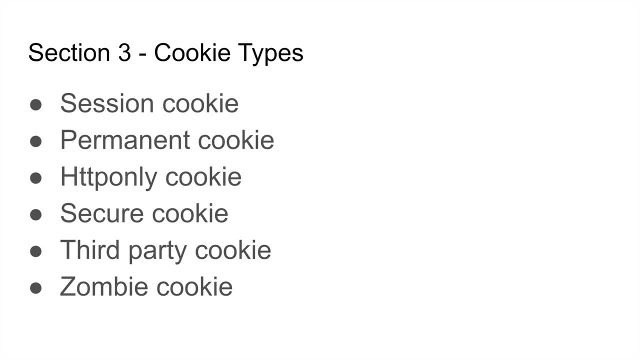 because if someone did a cross-site scripting attack on you and they cannot really read your session ID or token if it's set to HTTP only, because these guys are HTTP only and that means it will only get sent to the server, You cannot access it from documentcookie. 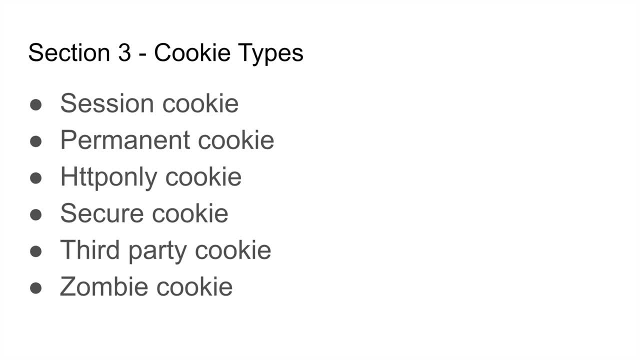 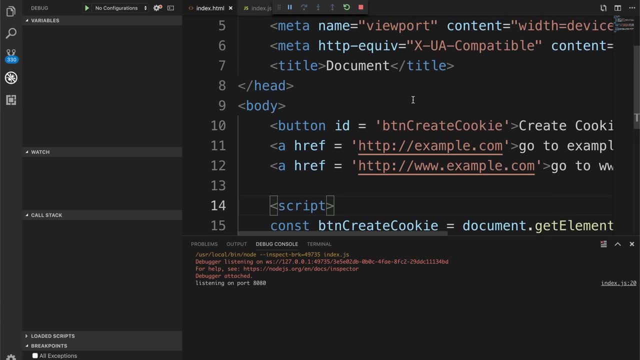 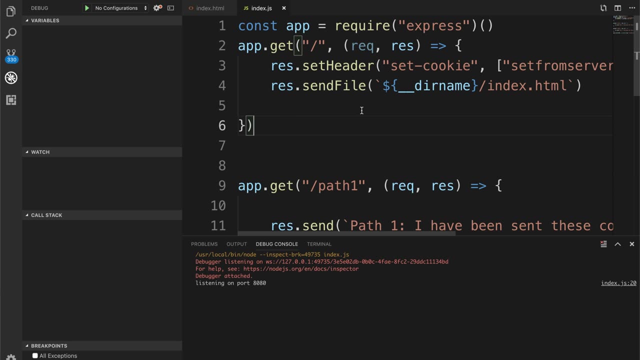 If you do documentcookie, you cannot see it right. But obviously if you go to the application, you cannot see it right. But let's show that, Let's show some example, guys, And close this. If I go to my indexjs. 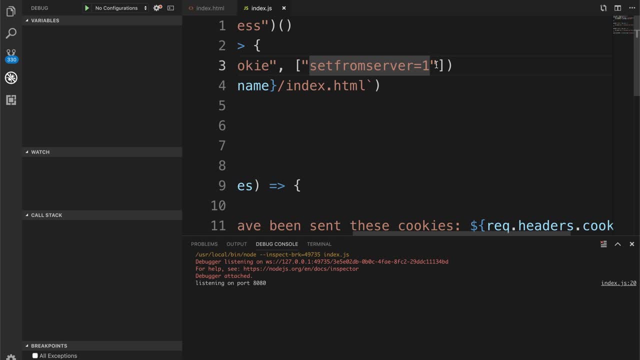 I'm gonna set sit from server here. I'm gonna make sit from server as an HTTP only cookie, right? So here's what I'm gonna do. I'm gonna make another one- This- no, js can't see this- equal one, right. 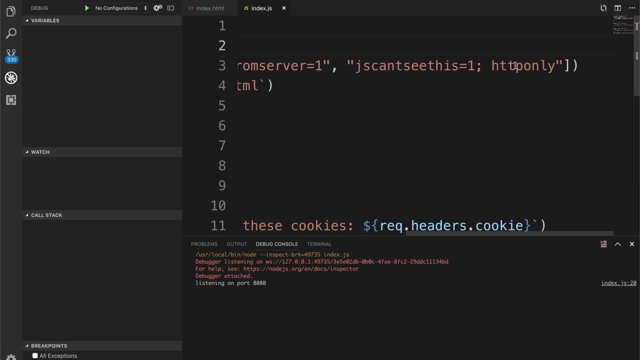 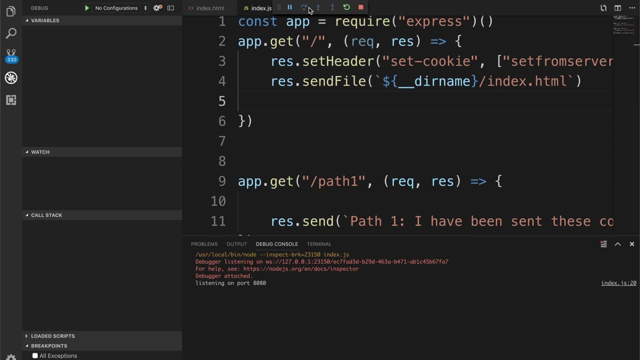 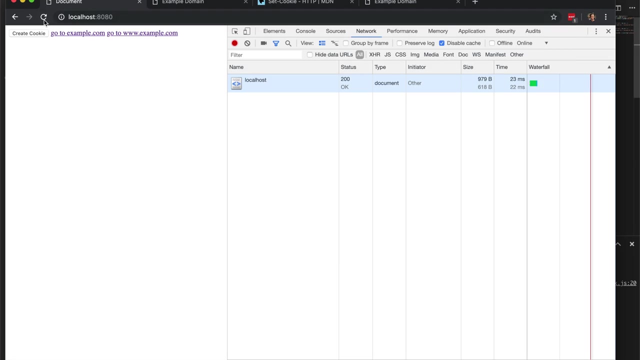 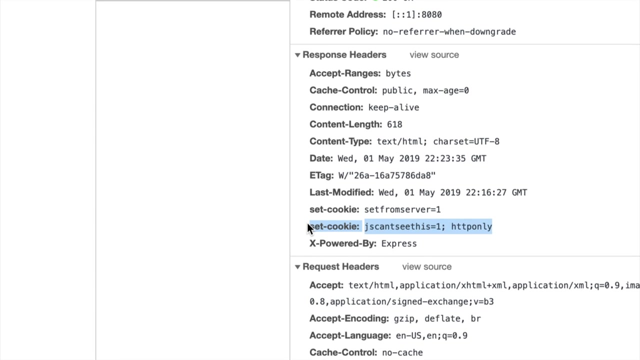 And we're gonna call HTTP only. I don't remember if it's called HTTP-only or HTTP-only. If you do that, then this one back rufferish- make the request. You can see that I have another sit cookie. 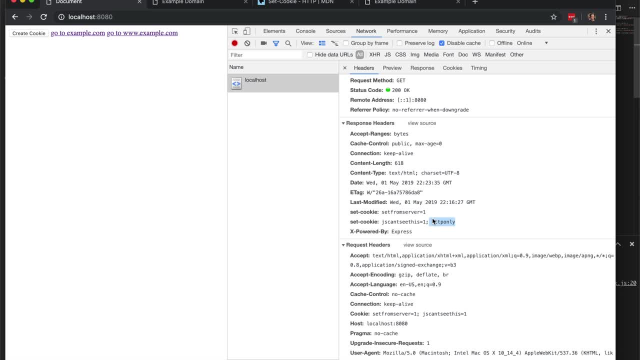 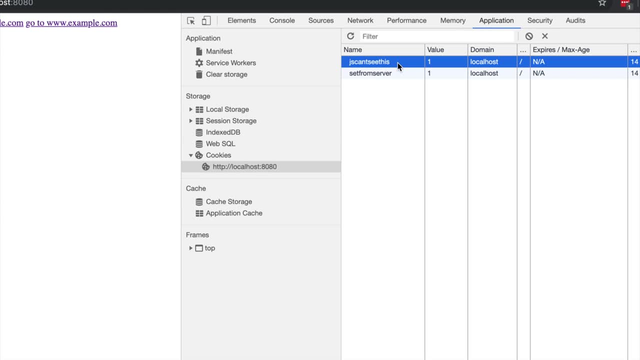 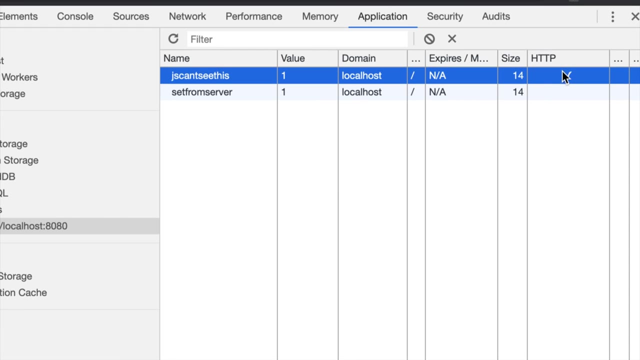 js can't see this. It's an HTTP only, right. That means if I do application, js cannot see this right. But here's a property that you need to see. guys here, Look at that HTTP. there's a tick. 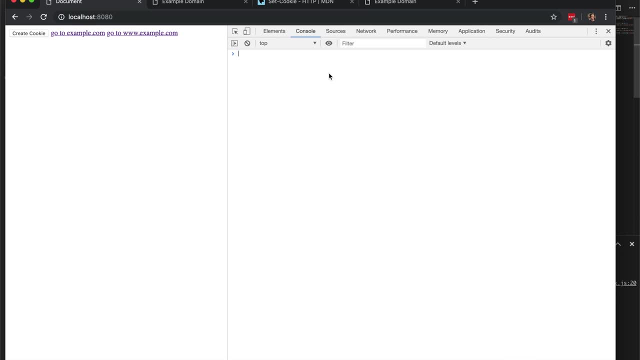 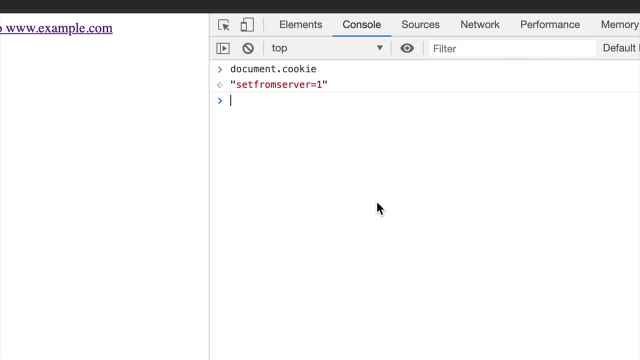 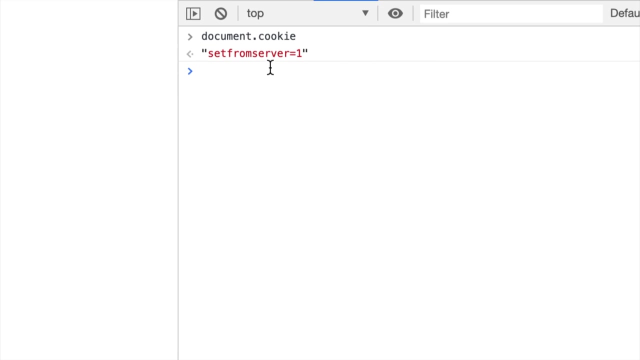 It means this is HTTP only. That means if you go to the client and you say documentcookie, guess what? That's what you get. You cannot see that one. If someone wrote some code to read, right? If someone wrote some code to read the cookies of the current browser, right? 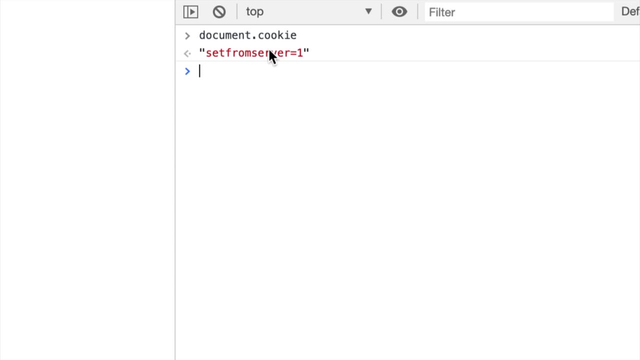 It's like they want to steal the cookie, which we will see in the last section. right, They want to take the cookie and send it somewhere else. They cannot, because it's an HTTP-only cookie. You cannot access it with documentcookie. 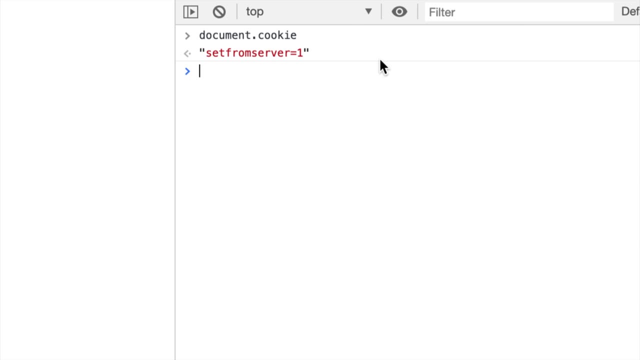 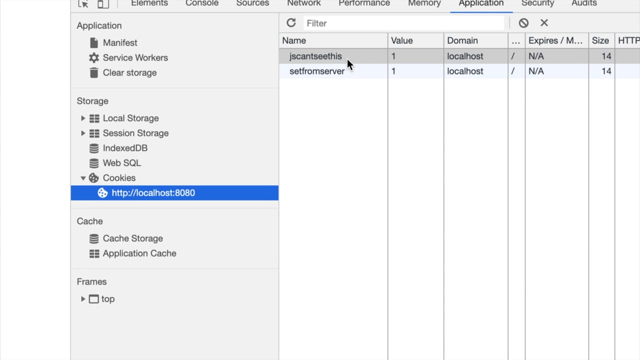 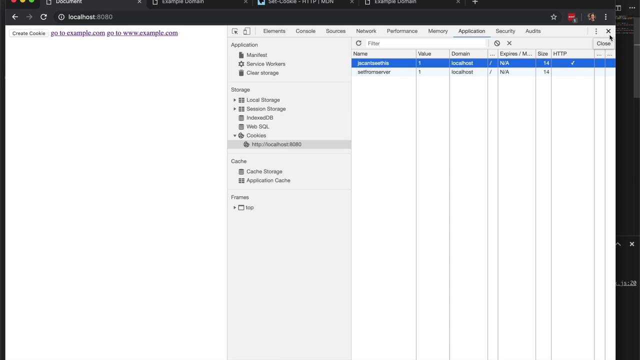 So there is no code that allows you to access this right. Someone will say: Hussein, I can already see it, It's right there, But this is different right. This is the console. It's a developer set. It will not be available for a hacker or someone, right? 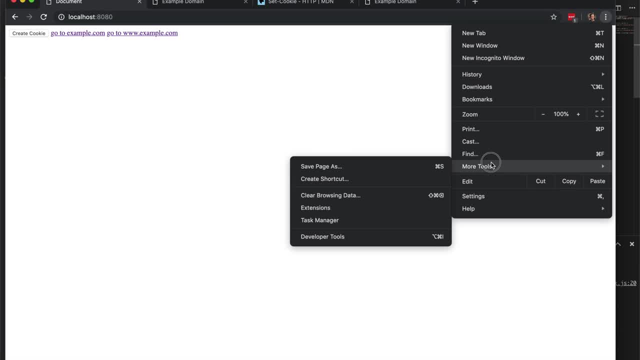 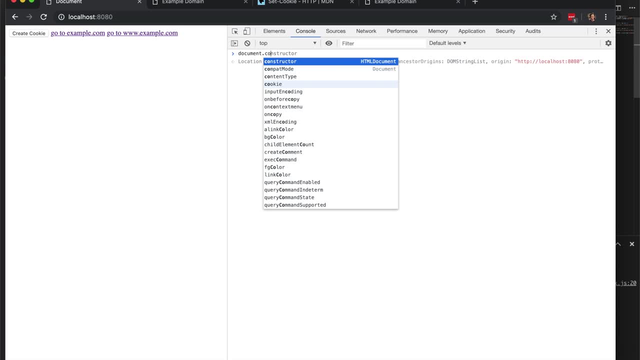 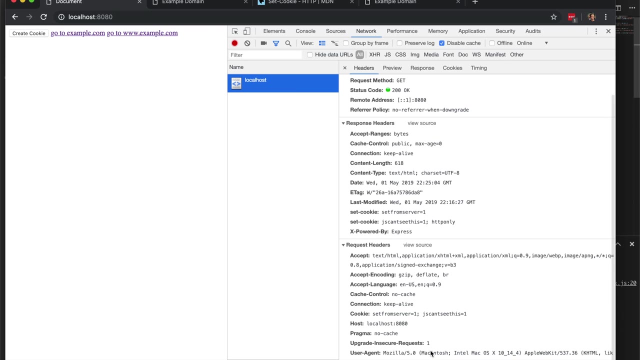 So you cannot write this code to access HTTP-only cookies. All right guys. So you cannot see that. So that's pretty cool guys. But guess what? If you do refresh or you make a request, you go to this. we are sending this puppy with a request. 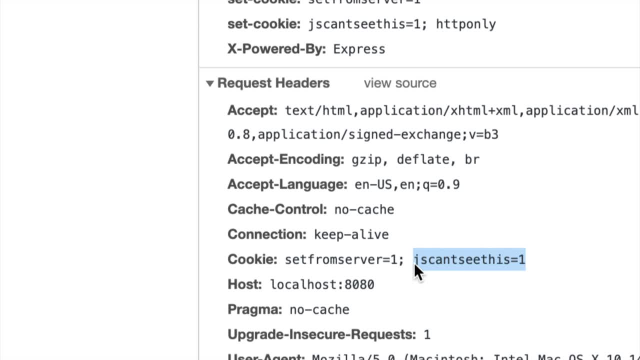 So we kind of see that We are sending this puppy with a request. We are sending it but you cannot access it from the JavaScript. So this is cool for kind of things like tokens, session IDs, things that you don't want people. 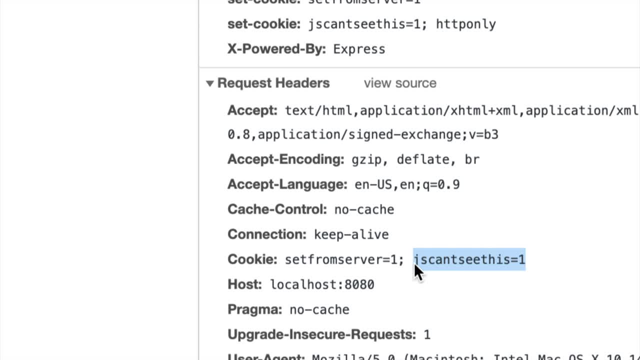 sniffing, But it kind of sucks. if you like building a game that relies on JavaScript, that you really need to read the cookie like scores, You cannot make scores with HTTP-only. That's just I don't know. It doesn't work. 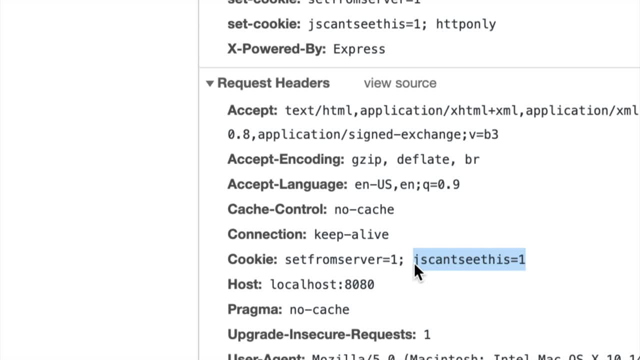 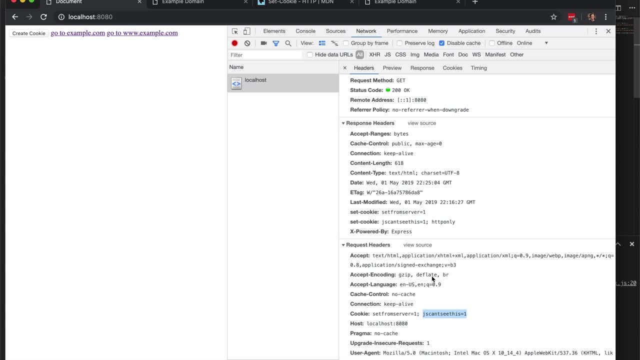 Because you need to display the scores. You need to display the score at some point right to the user, So you cannot make the score or the number of kills or whatever. So you have to make it into non-HTTP-only, if you will. 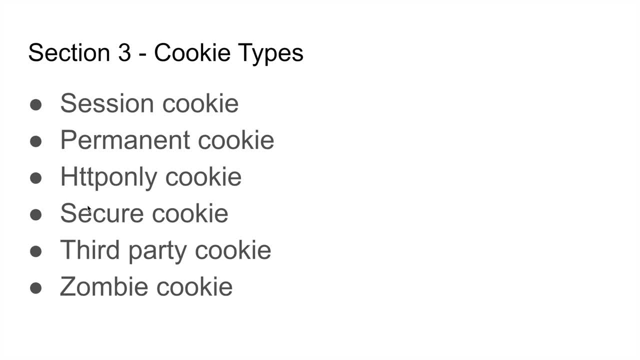 Secure cookie: Secure cookie- I'm gonna just pass through this. A secure cookie is another property that can put in the cookie, but it is only available for sites that are HTTPS, right. So secure cookies will only be available for sites that are HTTPS. 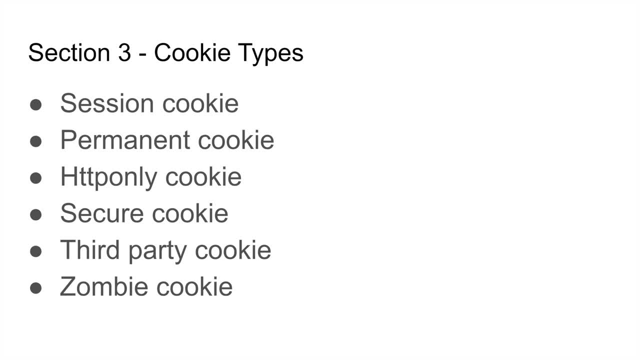 So secure cookies will only be sent to HTTPS domains. right, protocol. okay, That's the only difference, right? Third-party cookies: These are what the tracking servers uses to track you. okay, It's not really something special, guys, right. 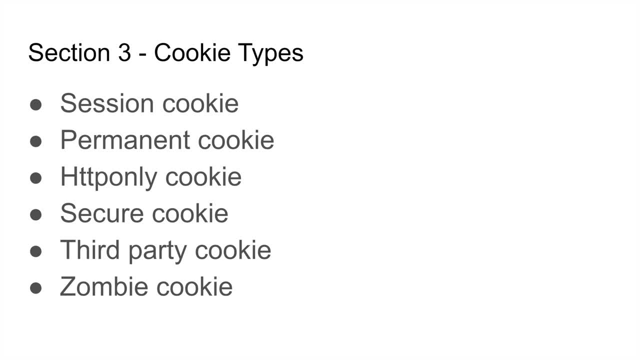 If you think about it, it's not anything special, It's just, It's just normal cookies, but they are available nested in your website. So here's an example. So you go to my blog, for example, and if I'm serving you ads. 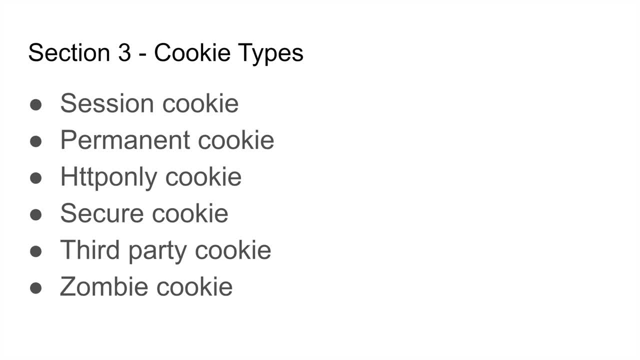